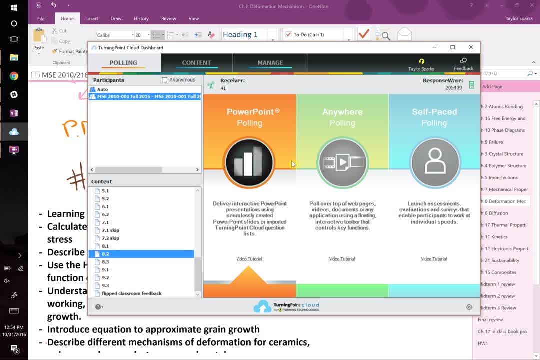 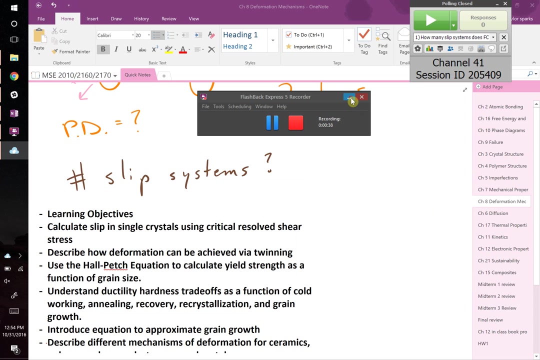 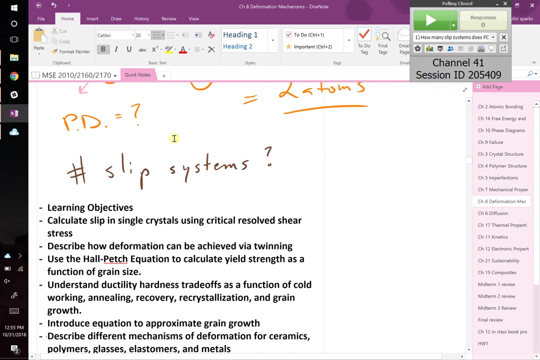 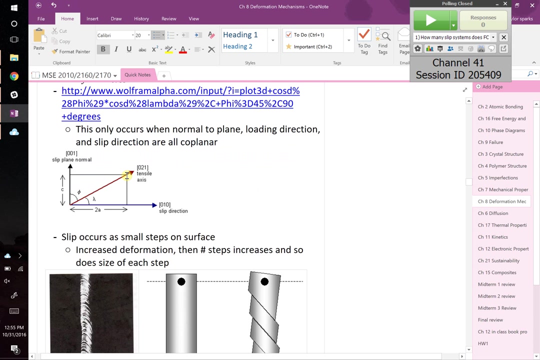 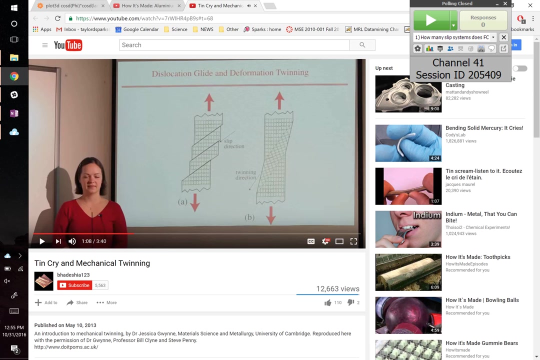 Thank you for watching. Thank you for watching Today. let's start with this brief video because it's pretty rad. Let me grab the mic, make sure it's turned on. Okay, you'll have to listen to this. That's the key part of this video is what you can hear. 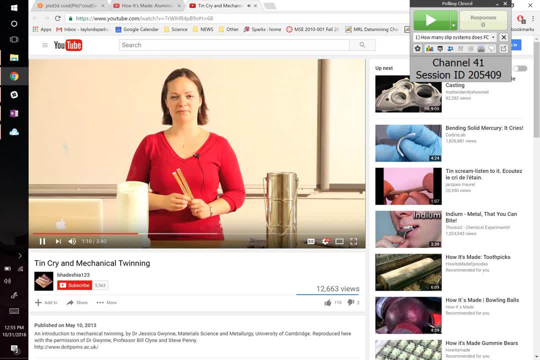 In this demonstration we're going to illustrate defamation of twinning using these two bars of freshly cast tin. So tin has a tetragonal crustal structure, which is a much lower symmetry of the raised metals, which makes dislocation motion more difficult and then favors defamation of twinning. 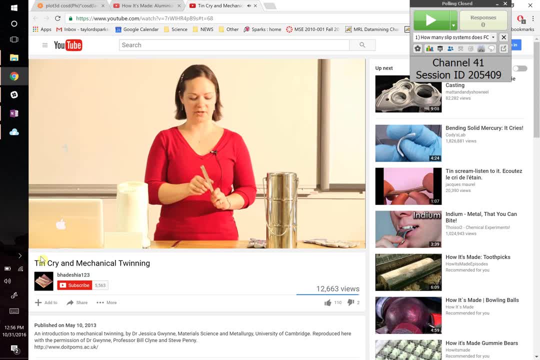 So I'm going to take one of these bars and I'm going to heat it up using freshly boiled water. So I'm going to leave that there for just a little while and in the meantime I'm going to take this bar that's just at room temperature and I'm going to bend it and I'm going to do that quite close to the microphone and you should be able to hear why in a second. 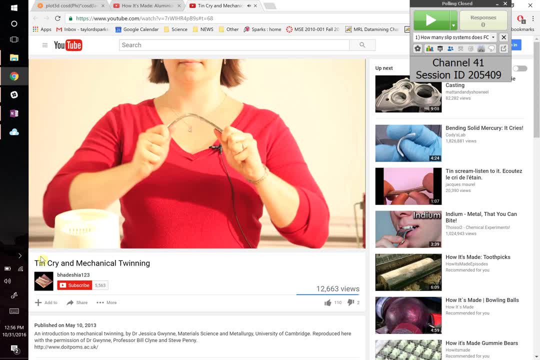 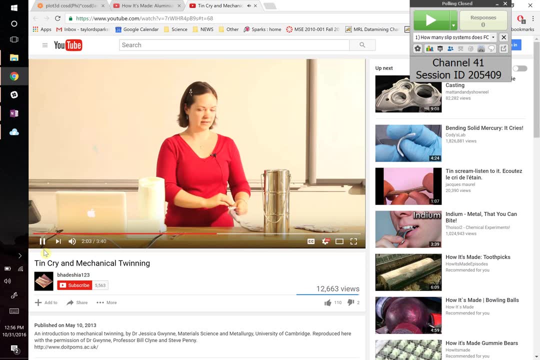 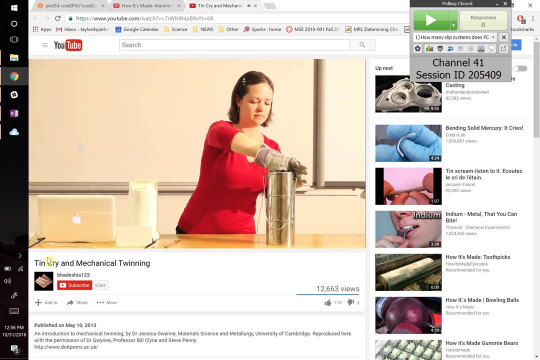 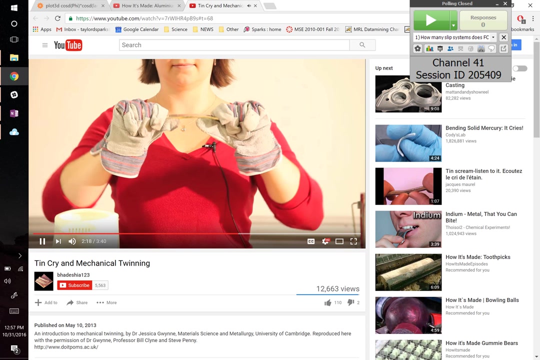 So now I'm going to take the one that's been heating up and do exactly the same thing to it. Okay, so the same material. only thing that's different is two different temperatures. One of them makes a really just awful noise as you bend it, and the other one's silent. 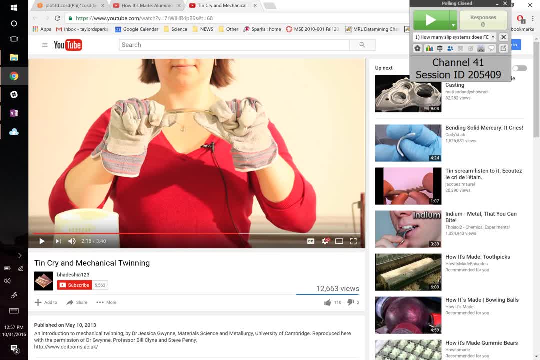 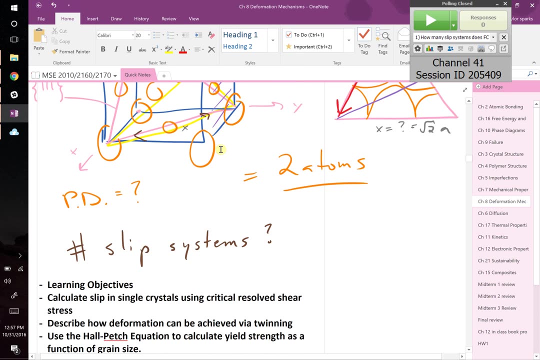 That just makes me crazy, Okay, Okay. So we're going to talk about what's the difference there. Why does one make that awful creaky noise and one does not right? So to pick up where we left off last time. so we'll get to that in about five minutes, but last time I said we'd pick up with calculating the number of slip systems in an FCC crystal. 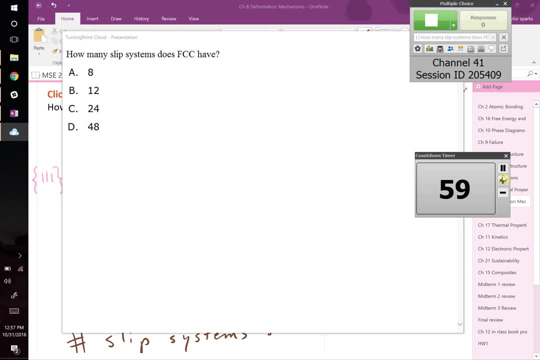 So I'm going to give you a. let's see how much time it's set for. We'll give you actually like a few minutes here, but I'd like you to calculate for an FCC crystal: how many slip systems does it have? 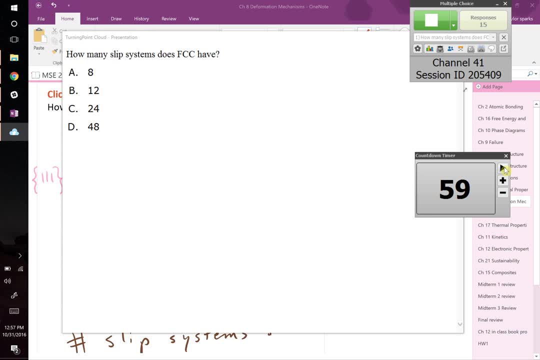 That means I want you to find out how many planes there are That are highest density, and then how many directions there are that are highest density directions. Now, if there's a direction going forwards and going backwards, that's still just one slip system, right? 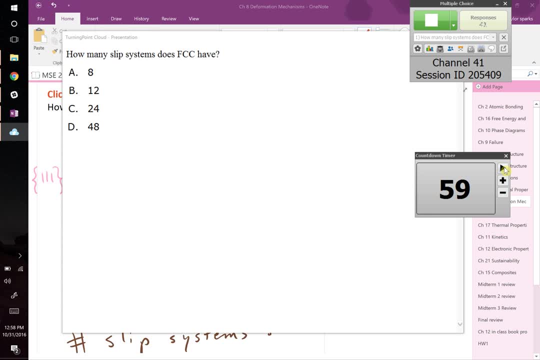 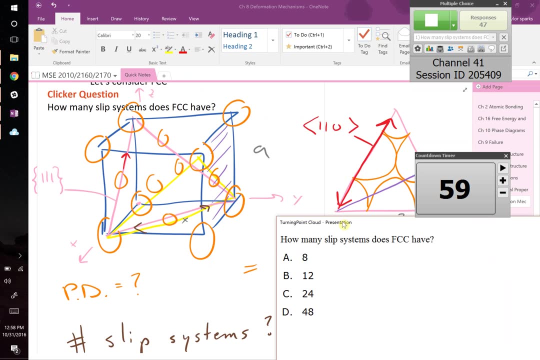 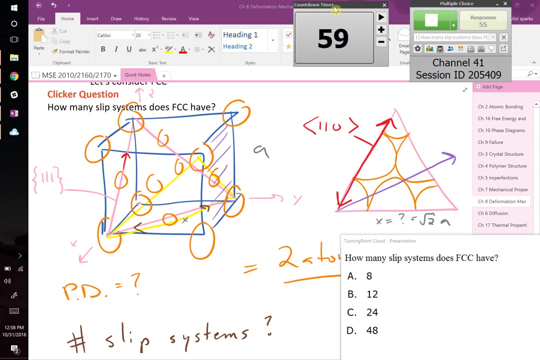 We don't count that twice, That's just one slip system. Okay, so with a partner, with whoever you want calculate whether it's A, B, C or D here. So one by two you can just take that, and if one of them is B, you get the other one. let's say A. 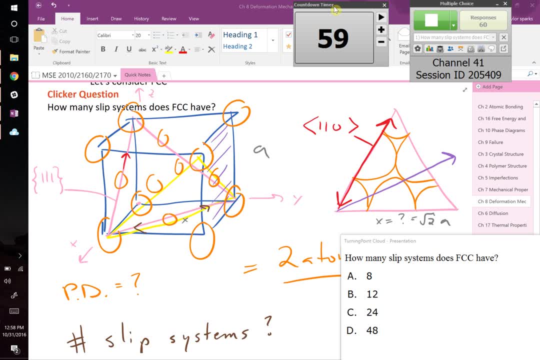 Like this. So that's one by two, Right? So this is how we're going to do it. So now, with O, we're going to use this one, So you're going to say: you know how many like the thing is here. 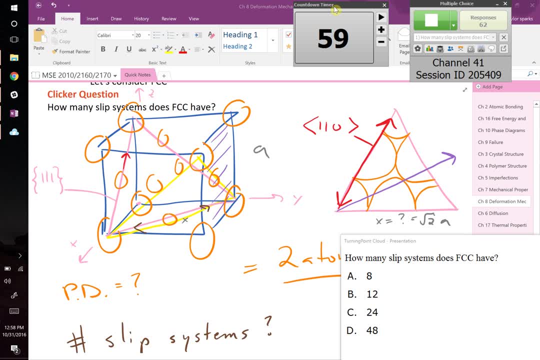 So you're going to give one of those numbers, right? Okay, And with O you're going to say: okay, how many of those numbers? right, I'll say, like you know, I like, I like to get those numbers. 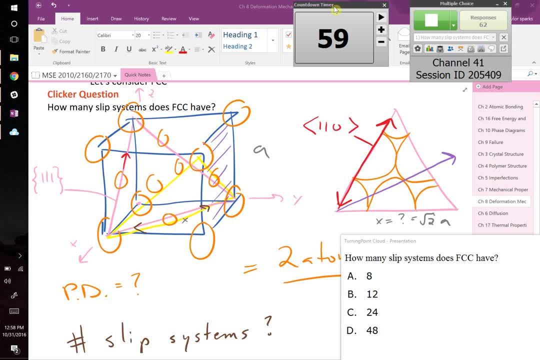 I'll say like that's you, That's you, Okay, All right. So I'll show you these numbers. You're going to say like that's my number, right? I don't think it's going to be straight down, but I think it's going to be like I don't know. I think it's going to be like I don't know. 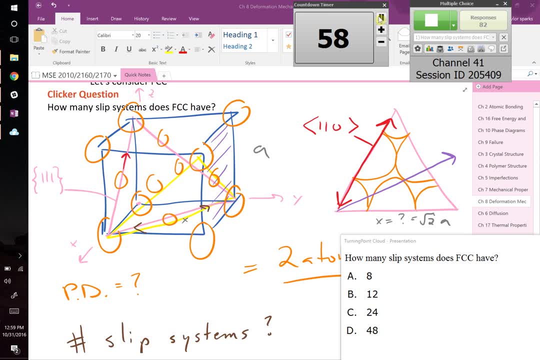 Okay, I'm going to go ahead and start the timer. So 60 seconds: get your answers in. Okay, here we go. Okay, here we go. Okay, 25 seconds to get this in. If you're still struggling, I think one way to think of this is to picture where these three sides of the triangle are. 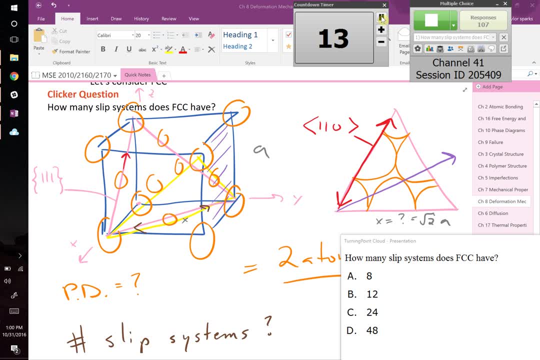 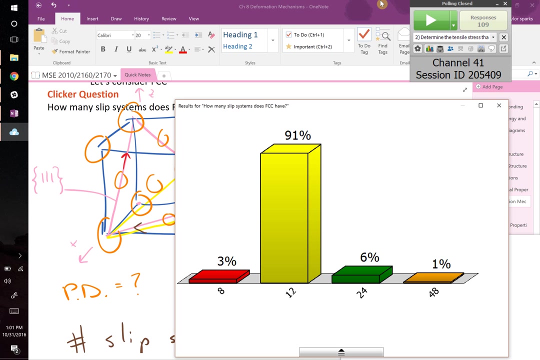 We know those are slip systems. Where would those be at on the cube And then add them up. Okay, let's hope you have your answers in A, B, C or D. People think, okay, overwhelming majority gets that it's B. 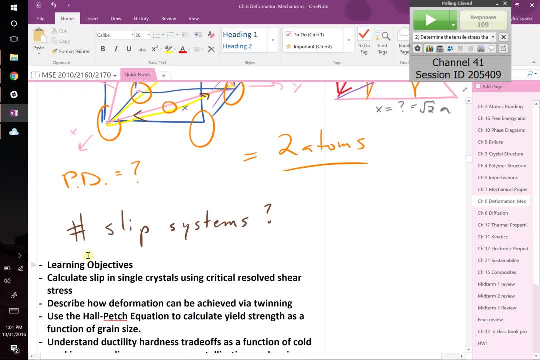 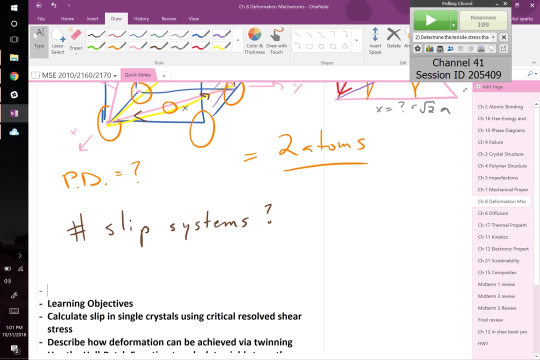 So for those that didn't quite understand why it was B, how do we understand it? Does somebody want to explain it to us that feels confident in their answer? Anybody? What do you think? Visualizing it is the key here. Let's try and draw it right. 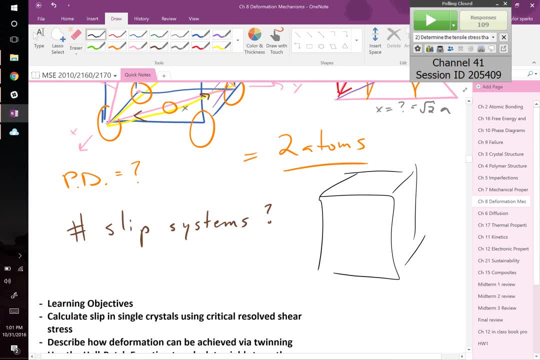 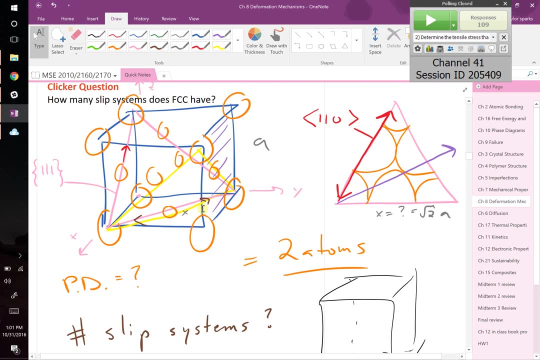 So let's draw a cube right. So a cube, just like a dice, has six sides And these things, these edges of the triangle, those cut across the faces of the cube right, So we could say that there are, like, on this bottom side, there's those two. 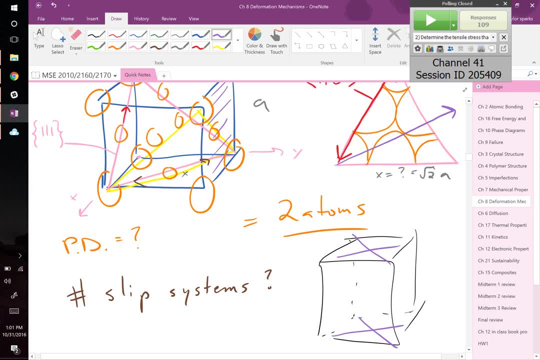 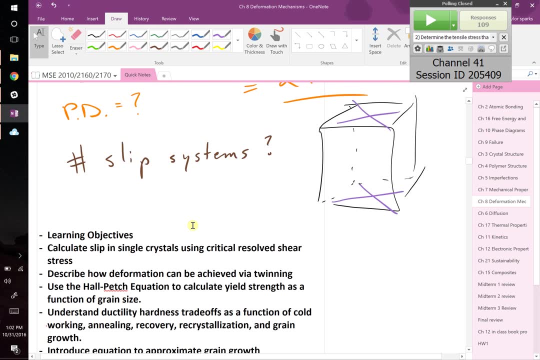 On the top side there's those two And there's six sides, right? So six times two gives us our 12, right? So that's where the 12 comes from here. Yeah, Matt, We'll do that in just a moment. 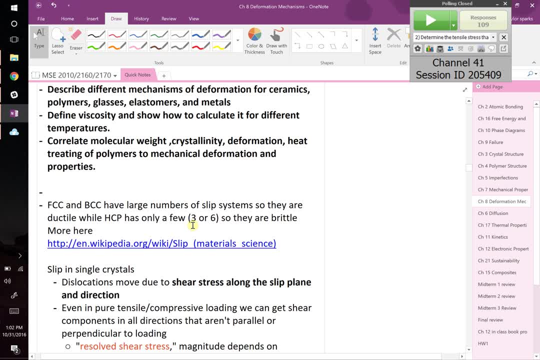 That one's harder to visualize. So maybe we'll do it for a homework question next week or something. Okay, I don't think I can get through it and still get through the material I want to cover for today. Nobody stone Matt, please for doing that. 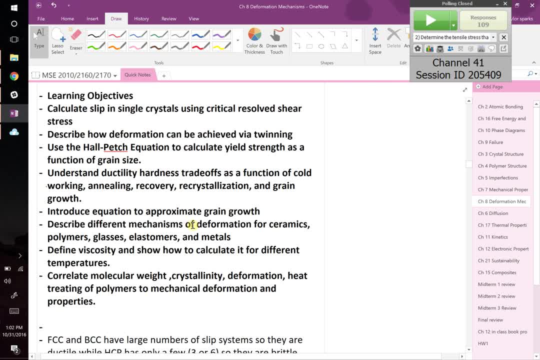 Okay, Okay, so let's talk about the learning objectives for today. We're going to talk about slip and single crystals. We'll actually calculate it. That's where we left off last time. We'll describe how you can deform via both dislocation, motion and twinning. 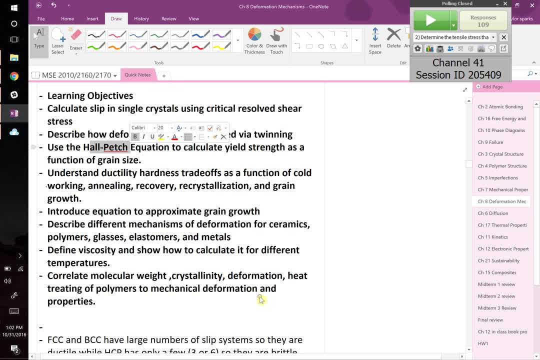 And that goes back to the video we started class with. We'll describe what is Hall-Petsch. It's one of these, like early fundamental material science equations And how we use it to calculate yield strength as a function of you know, grain size. 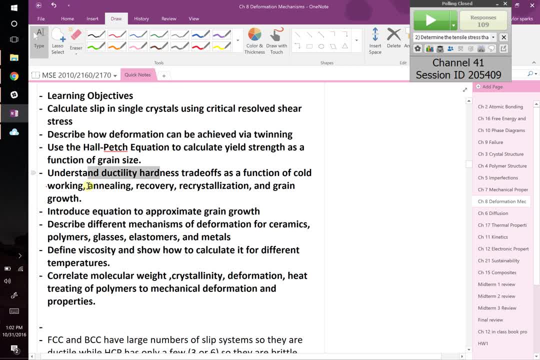 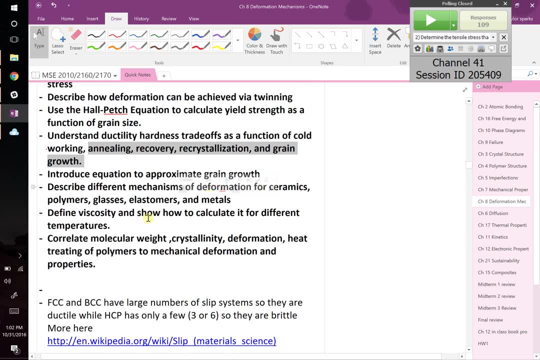 We'll talk about ductility and hardness. We'll actually calculate it. We'll introduce these important concepts of annealing, recovery, recrystallization and grain growth. We'll talk about deformation in ceramics, or the lack of deformation in ceramics. 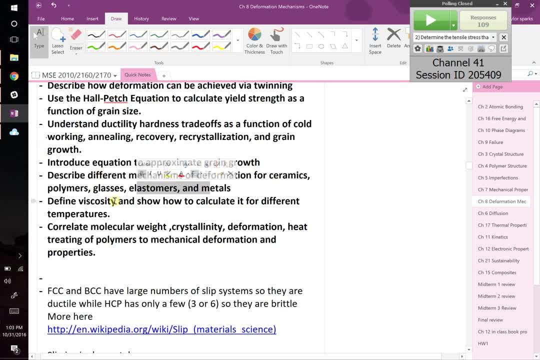 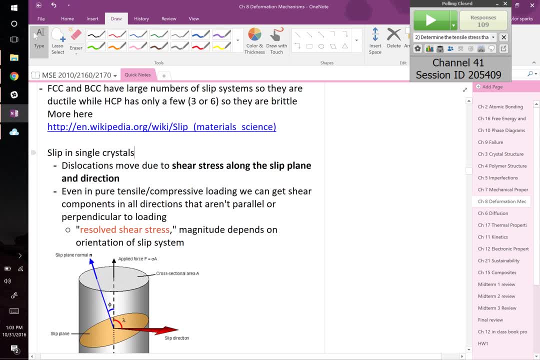 But we will talk about how glasses, elastomers and metals deform. If we have time, we'll get to viscosity And we'll even tie it into molecular weight and crystallinity of polymers. Okay, So we left off last time. 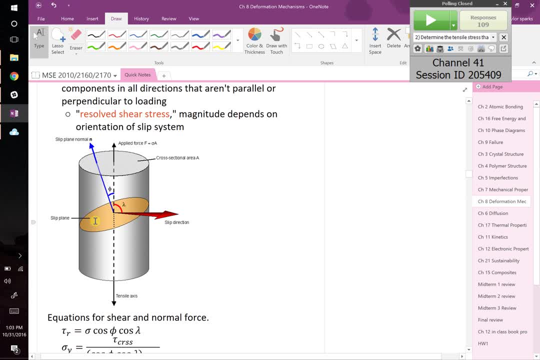 We said that If you have a single crystal, imagine this big cylinder is a single crystal. right, It's a giant, giant like crystal of silicon. They actually make them huge, right They're? they're 12 inches. 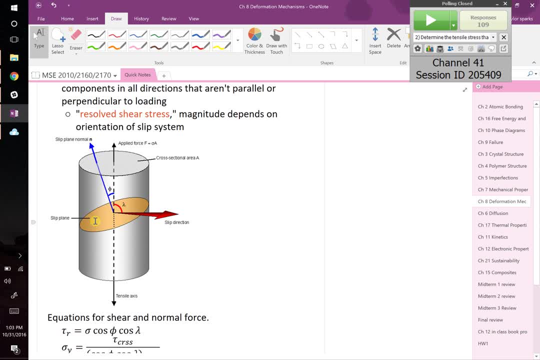 They even make them 15 inches wide now and like 12 feet tall, All perfectly oriented in one direction all the way through right. So if you take that and you pull on it, what I've said in class is that you're only going to get motion along your slip planes, right. 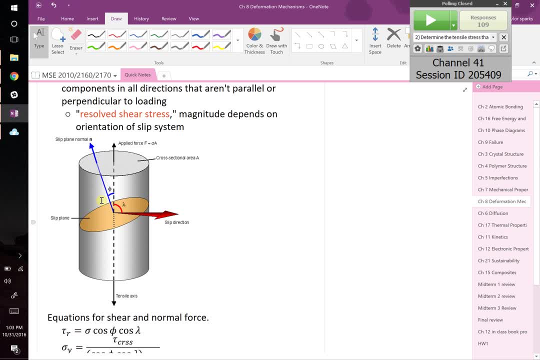 So on your slip planes and in the slip direction. So it has to happen on your slip system. but what you don't know is whether or not the way that you grew your crystal, with its orientation, if it's going to cooperate with you trying to deform it. 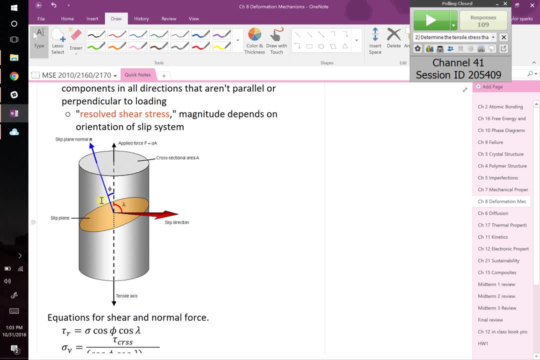 So, for example, in this picture, if the slip direction has to happen along this red direction here, but you're pulling it not, you know, parallel to that red direction, how do you get it to slip? Well, we said, all right, you have to take the force that you're applying to it. 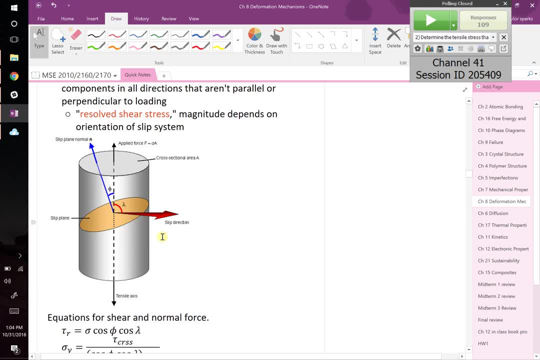 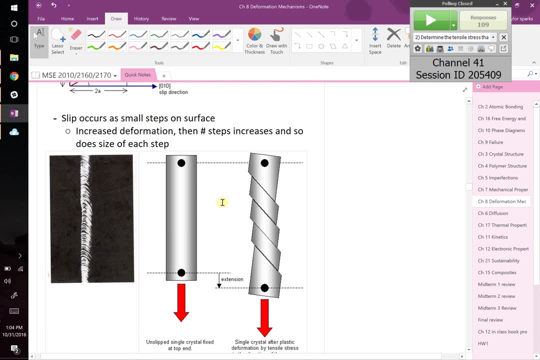 which is going to turn into a stress, and you have to break that stress up into components, right, And so there'll be a resolved shear stress, basically along this direction. So Matt at the end of class last time said: well, does that mean that when you pull it? 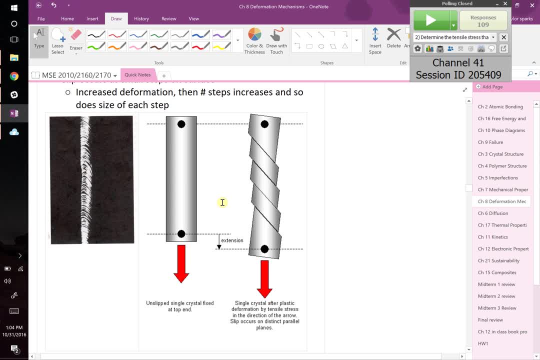 you're going to get a bunch of series of small slips. That's exactly what you're going to get, right? So this is an actual sample of a single crystal that they pulled, And you can see that the slip planes would be sort of like this: here and the 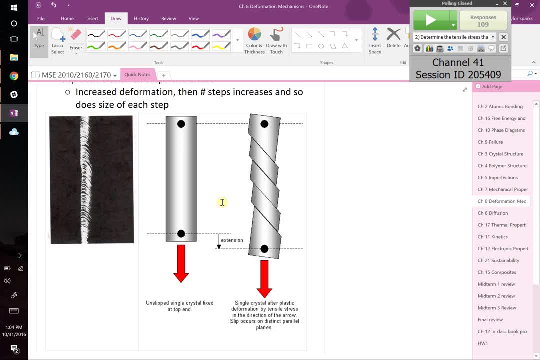 direction was that way right. So as they pulled it it did slip a little bit like that. So the overall deformation is a vertical one right, And this one relative to this one, but it doesn't achieve it by stretching the atoms out. 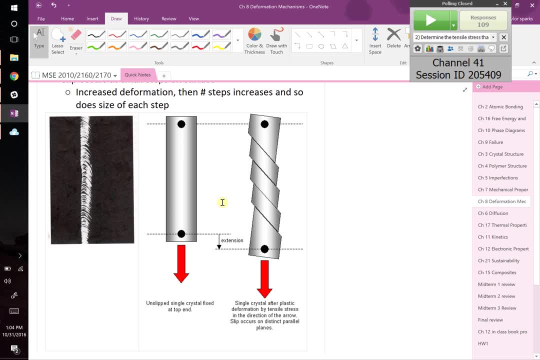 They actually have to slide past each other along whatever slip system was right. So if you grew this crystal in a different way and the planes were oriented differently, then you're. your little kinks here would be slightly different spacing right, But the principle still stands that you have to have slip along there, unless you 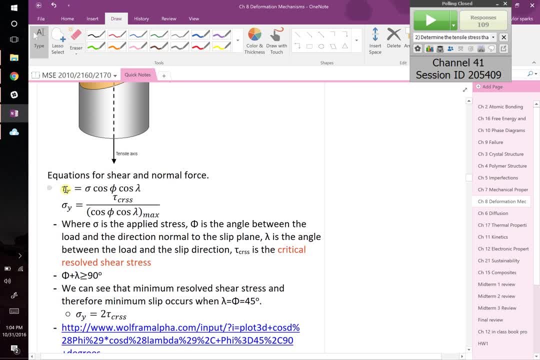 have twinning. We'll get to twinning in a second, So how do you calculate it? All right, Our resolved shear stress, that's tau r, is going to be equal to the stress that we apply sigma multiplied by the cosine of phi, and phi is the angle between the normal of 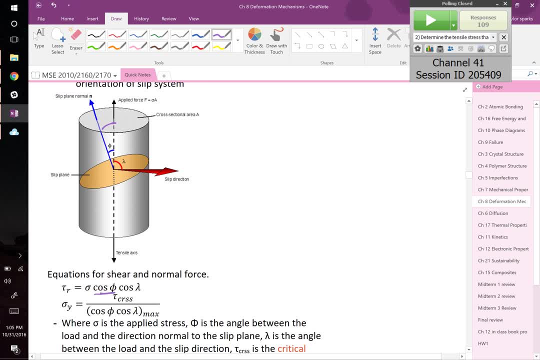 the slip plane and the loading direction and then cosine of lambda, And lambda is going to be the difference between the loading direction and the slip direction, right? So we need to calculate those two angles so that we can take the cosine of them to figure. 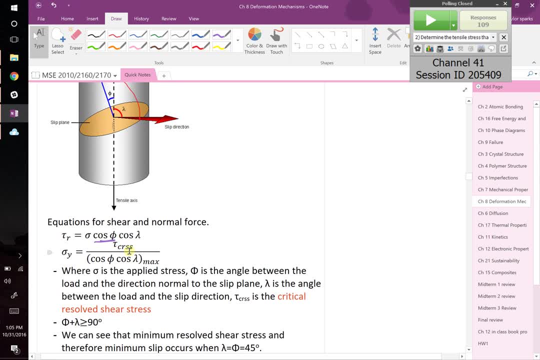 out this equation right? Therefore, since the critical resolved shear stress is a materials property, it's going to be a materials property, right? This one's known The tau CRS. that's the critical resolved shear stress. We would like to know. 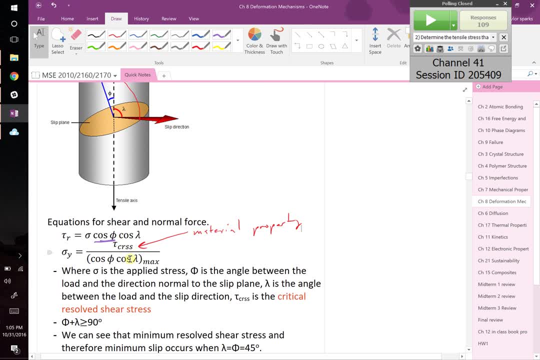 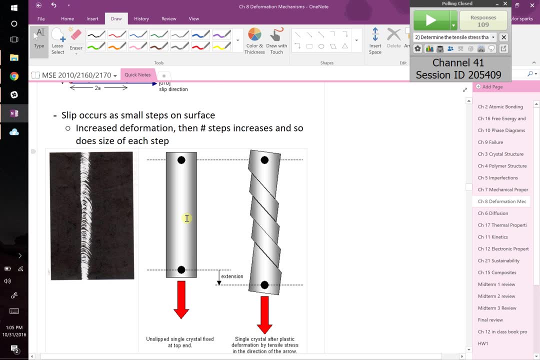 so, as a function of whatever this tau CRSS is for a given angles, what stress will cause this thing to start slipping right? So when they started pulling on this thing here, probably nothing happened when they were pulling on this one until they hit a. 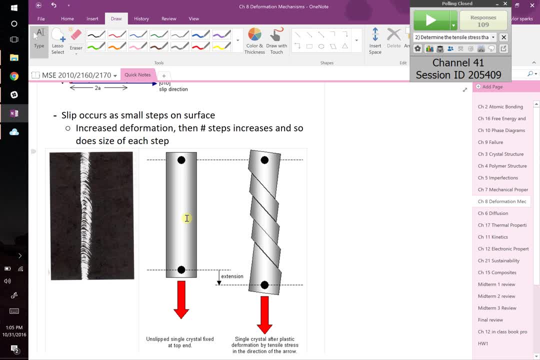 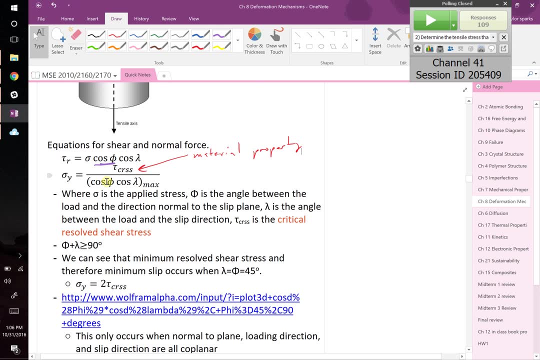 certain stress, the yield stress, when this thing did start to slowly start sliding past each other. So how do we calculate how big that is? We use this equation right here, right Now. one last catch here is that these angles can't just be arbitrary. 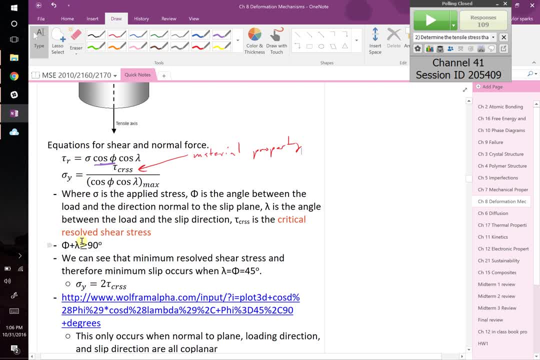 They can't be anything. In fact, we know that a phi and lambda have to add up to be at at least 90 degrees. Why? Why does phi and lambda have to add up to be at least 90 degrees? This is oftentimes hard for students to grasp. 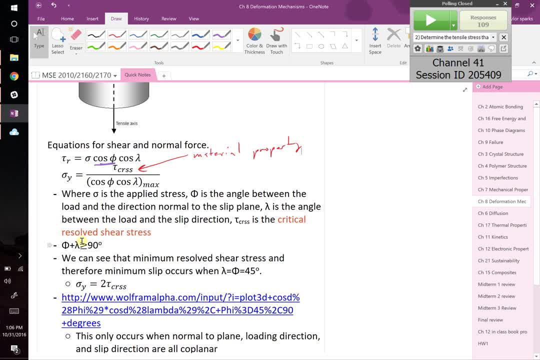 So let's imagine, in this plane down here, this is the slip plane, right? So it's maybe sitting on this table, So the table is where the slip plane is going to happen, right, And then the slip direction might be wherever it's pointing, right? 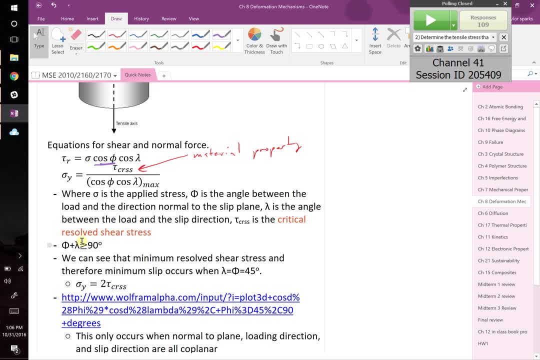 So right now the slip direction would be towards Ryan, but it's along this plane, right, Fair enough. Now the normal to the slip plane is this thing: It's pointing straight up from it. right, It has to be the normal. 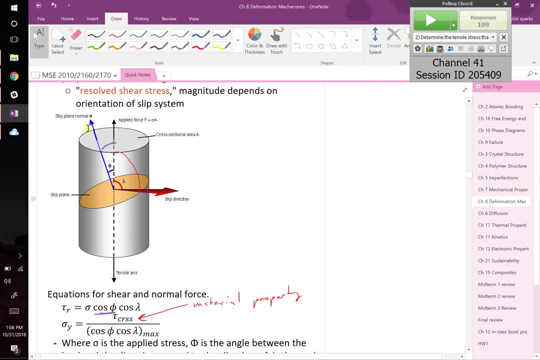 Right. So, going back to our picture, we needed this blue line. That's the slip plane, normal, right? That's this one And then the red line. that's where this thing's pointing. So these, we know, obviously have to be 90 degrees right To each other. 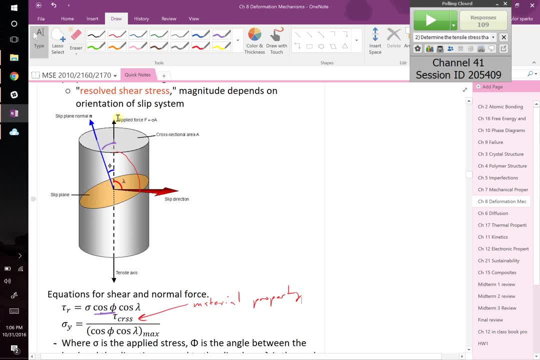 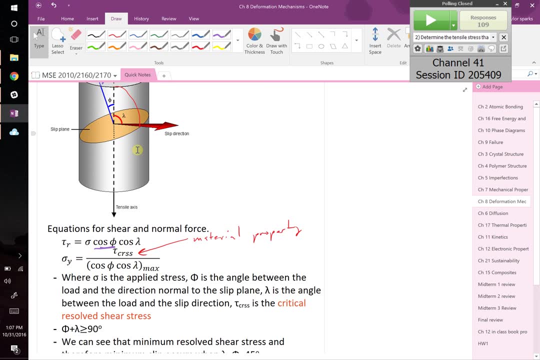 So the question is: why does when you apply a force? why do these have to be at least 90 degrees? Well, because, at best, if now we introduce another vector here, now, this is the way we're pulling it. Let's say that I'm pulling it in plane of these two things, right? 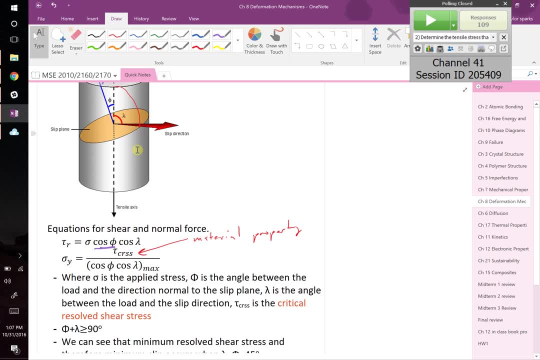 Then it still has to add it to be at least 90 degrees, right? 45 from hang on to this, checking on, 45 here maybe and 45 here. So at least it has to be 90 degrees, but it can be more because this could be like that. 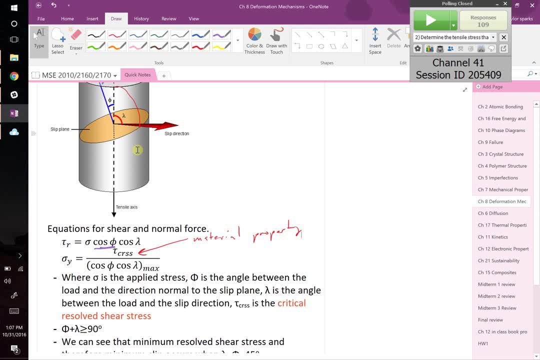 but I could be pulling on it like that, And so then you could have greater than 90 degrees when you were to add those two angles up. right, That makes sense. Are there any questions on that? Okay, That's hard to grasp sometimes. So because of that, 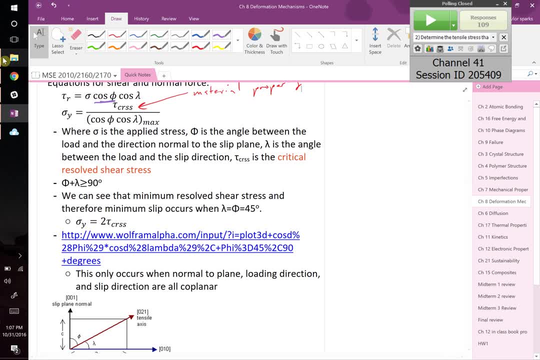 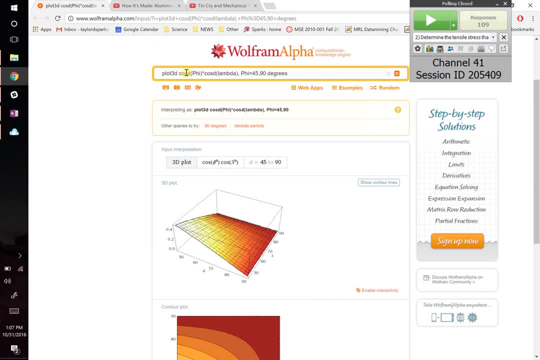 they have to be at least 90 degrees. At what point will they be 90 degrees? They have to be the largest. So we can plot it right And it turns out if you plot right here. so we're plotting in 3D the cosine of phi times the cosine of lambda in degrees. 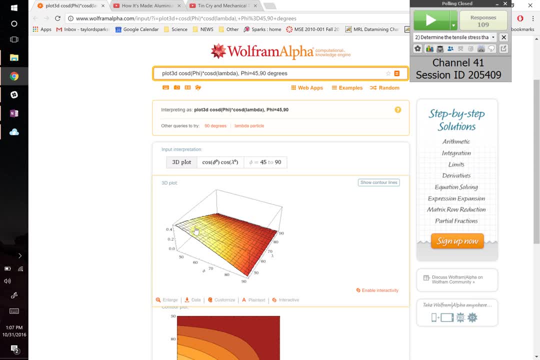 we're going to plot it from 45 to 90. And we find that the largest value there corresponds when both of them are equal to 45 degrees. Okay, Which means this is our slip system, right, If you want slip to happen? 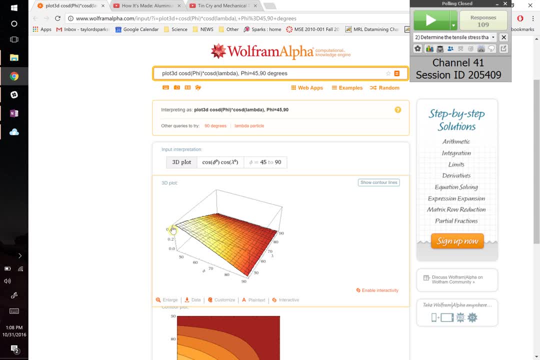 the best case scenario would be to have this lined up in it, right? If it's, if it's all coplanar, then you'll have the highest likelihood of slip. This will be less likely because your resolved force on it is going to be a. 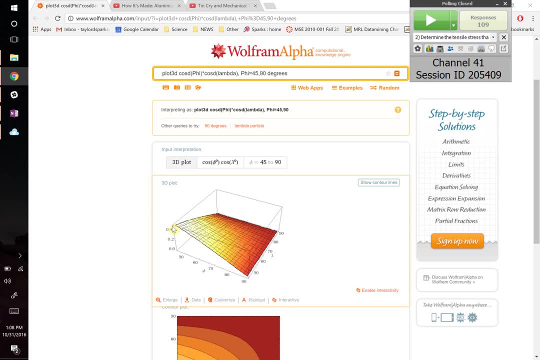 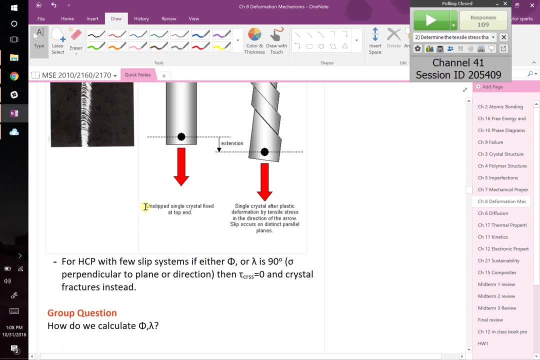 little bit less right. That's all that means, Okay. So what we really need to figure out, then, is: how do you calculate these angles? That's what it really comes down to right, Because, ultimately, I'm going to tell you that it's loaded along some direction. 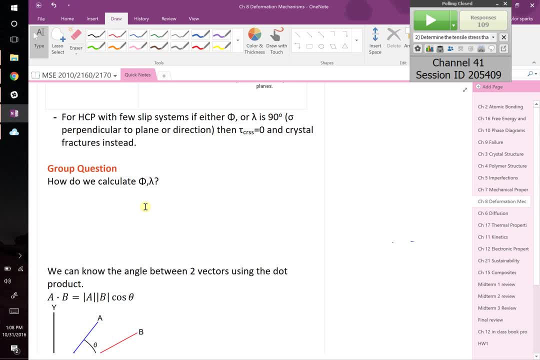 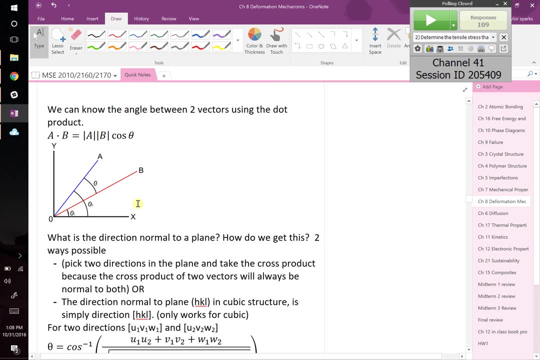 The slip system is along these planes. How are you actually going to turn that into angles, right? So we know how to calculate these things. Um, and we do so with something that you did back in geometry or trig at some point in your math career. 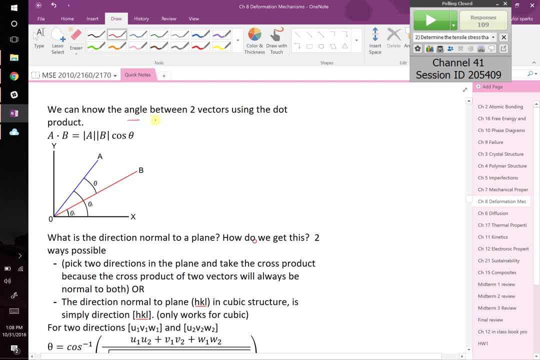 you would have seen this, that we can figure out the angle between two vectors by using the dot product, right? So the dot product of two vectors, vector a and vector B, is going to equal the length of vector a times the length of vector B, times the cosine of the angle between them. 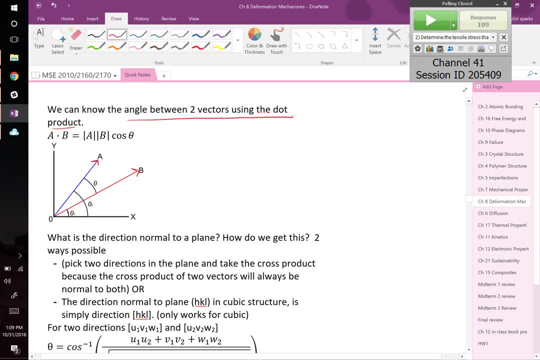 right. So if these are the two angles that we're trying to figure out on a question- and we need to- or sorry, those are the two vectors, So we need to figure out that angle- We can just, we can just apply the dot product rule. 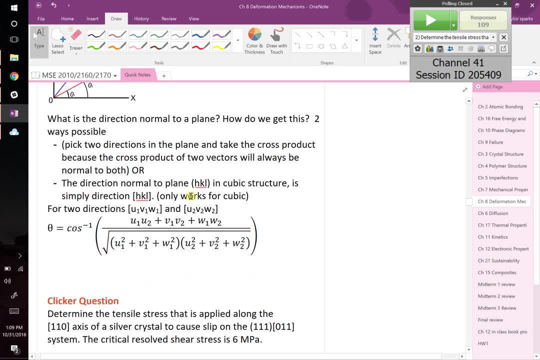 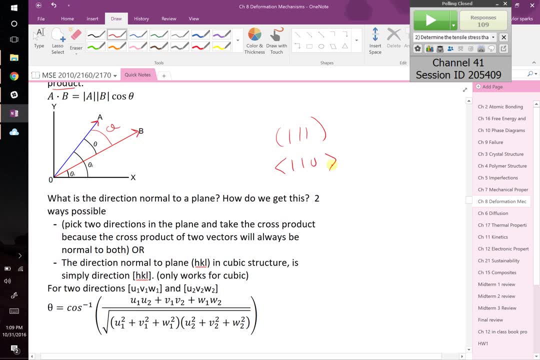 Okay, Now how do we figure out the direction normal to a plane Like, let's say that the slip system is the one, one, one plane and we said it's along the one, one, zero family of directions? How do we figure out the actual planes associated with that? 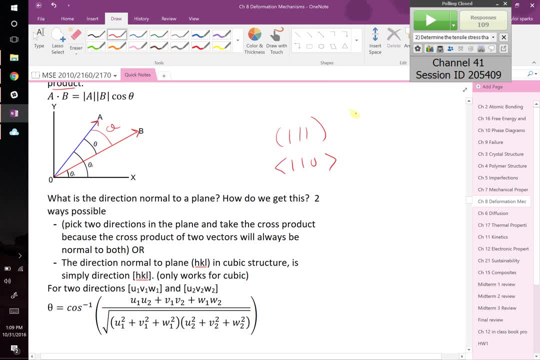 First we have to figure out what. what direction is normal to this plane? right, So normal to that plane? that's the perpendicular sign. It's actually this direction, one, one one, in the cubic system that makes our life really easy. It means, if this plane at this table is the one one, O plane. 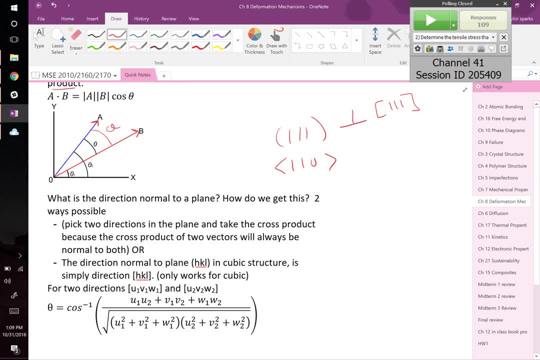 then the normal is just the one one: O direction. that only works in the cubic system. right, I won't give you anything harder than the cubic system in this class and your other courses You may have to do that right. Hexagonal or tetragonal. 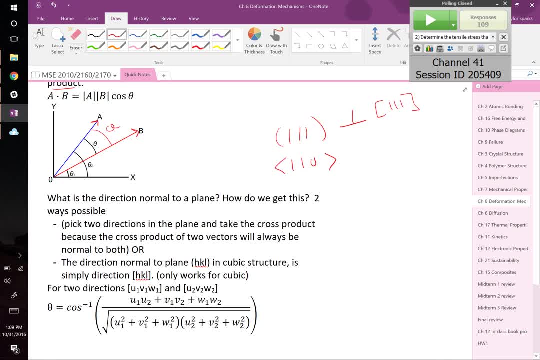 It doesn't work like that, but in the cubic system in this class, it makes it easy. if I give you the slip plane, what's the normal to it? Same thing as a plane, but now, instead of writing as a plane, you write it as a direction. 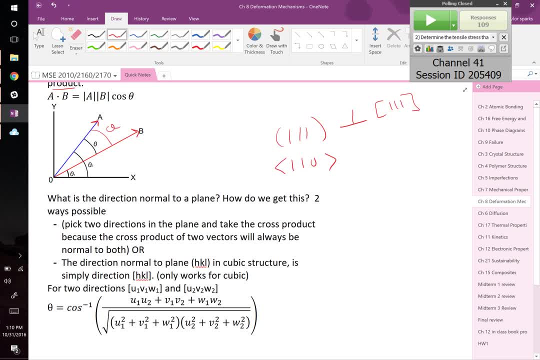 Okay, Any questions on that? So let me ask this: If it wasn't cubic, if it wasn't, if it was tetragonal or some other system, how would you figure out the normal right? How might you figure out the normal to a plane? 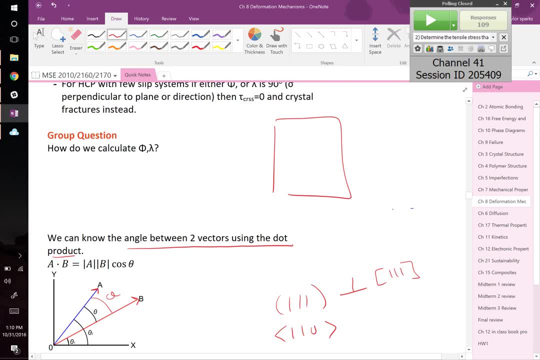 First of all, do we need to convince ourselves that it's actually normal? Imagine you've got your, your cubic crystal right. So we said that the one one, one plane is this one. So is the one one, one direction normal to that? 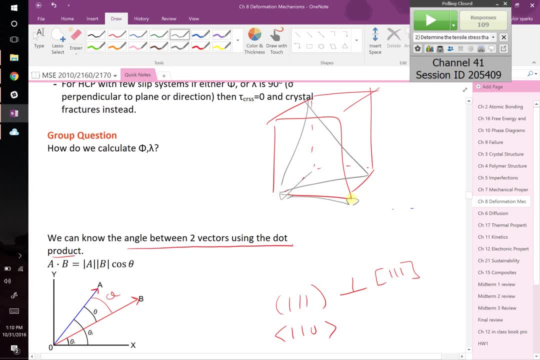 Sure, Because one one, one direction. that means we go one this way, we go one that way, we go one that way. Therefore, our overall direction goes from this one to this one, This corner up to that one. So sure enough. 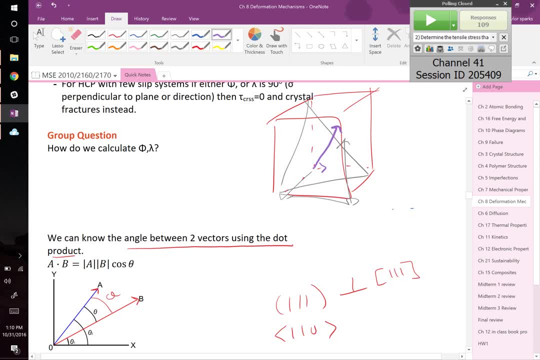 that thing will be normal to that plane, right? How would you figure out if it wasn't cubic? and we don't have this handy rule that makes our life easy. Any ideas? Yeah, How would it? how would it work? How do you know that that would give us something normal. 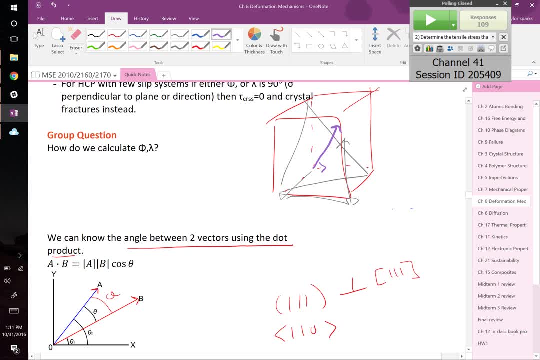 So basically, cross product says you have vector one and vector two. If you take the cross product of those, you'll always get something normal to it. So all you'd have to do is say, all right, in this plane I know maybe what this direction is. 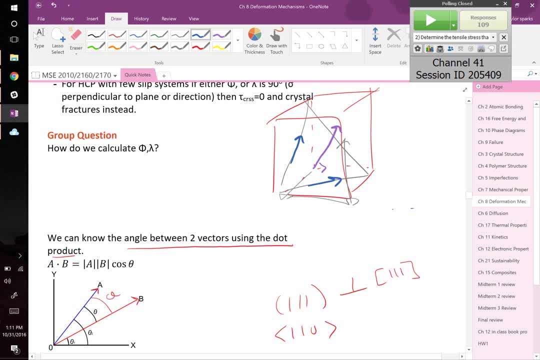 I know what that direction is. I could take the cross product of those two and I would get something normal, And that works for cubic as well. but we don't have to use it because it's easy. Whatever the plane is, same numbers are the direction. 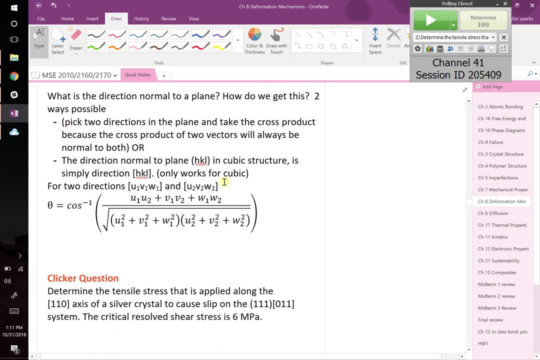 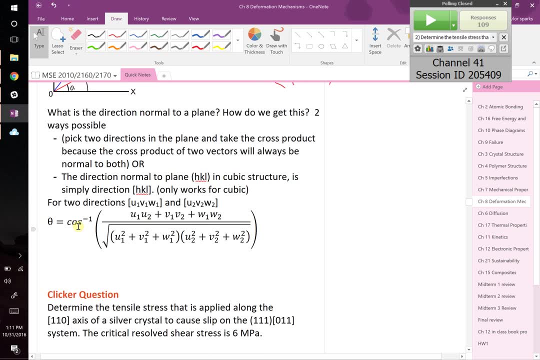 Okay, Um. so if you don't remember how to do like length of vectors and doc product, I've written it out here that the angle would just be equal to the inverse cosine of all of that jazz, where you one V, one W, one U, two V, two W two. 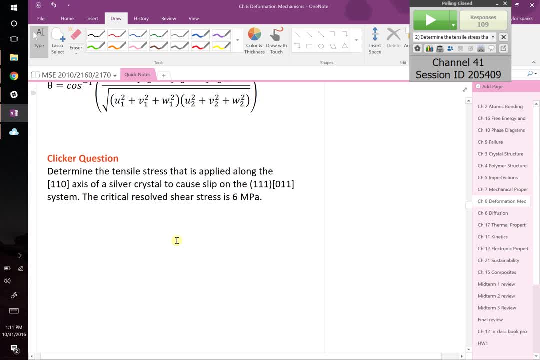 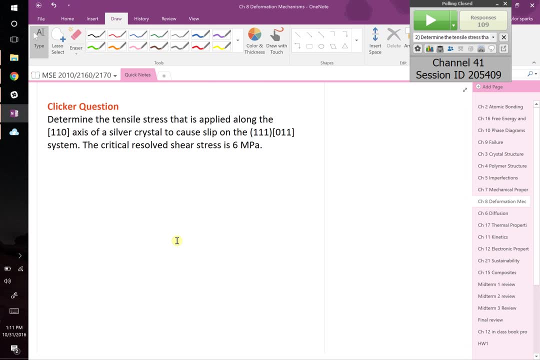 are your two directions. You're trying to figure out the angle of. So, with that in mind, let's figure out this next clicker question. So it says the following. it says: determine the tensile stress that has to be applied along the one one O axis of a silver crystal in order. 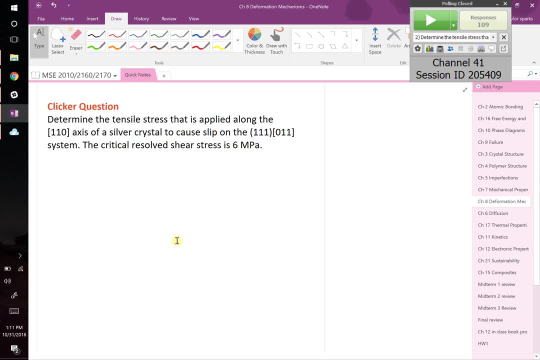 to cause slip on the one, one, one O one one slip system If the critical resolve, shear stress, is six mega Pascals. So let's remind ourselves of the formula here before we start. We know that Tau CRSS is going to be equal to the applied stress times. 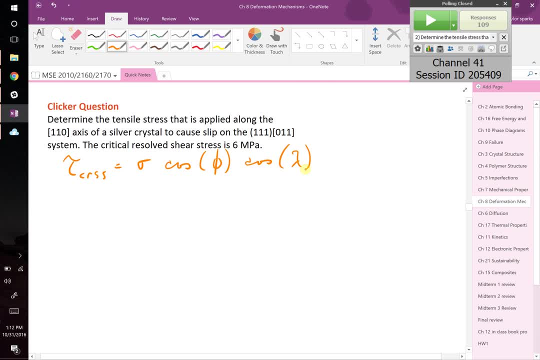 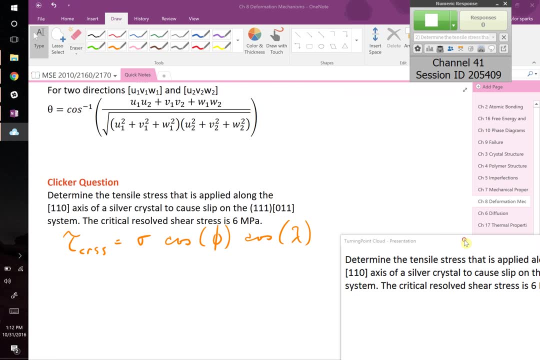 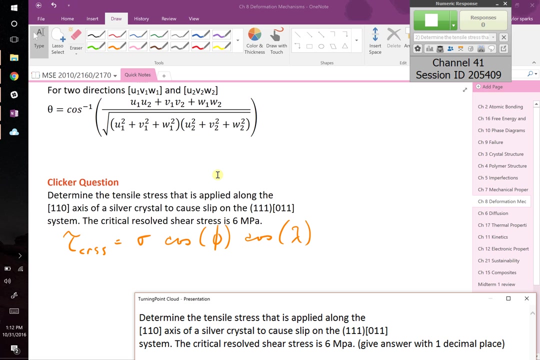 cosine of fee times, cosine of Lambda. Okay, And that is our equation for the angles. Okay, So I'd like you to give your answer within one decimal place and give the answer in mega Pascals. I'm sure Anybody need help getting started. 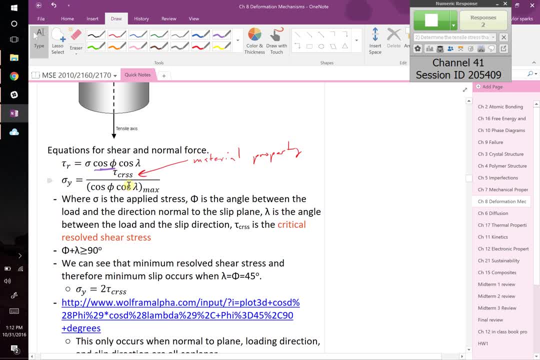 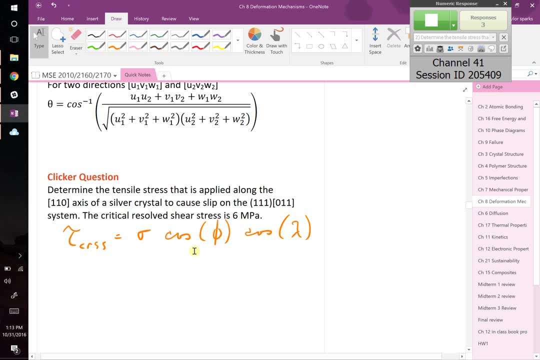 It's just rearranging the one that I did give you. It's this, just that one. It's just rearranging it. So from this formula you can solve it. We know that The balance volume has, while the yes, So you don't need help getting started. 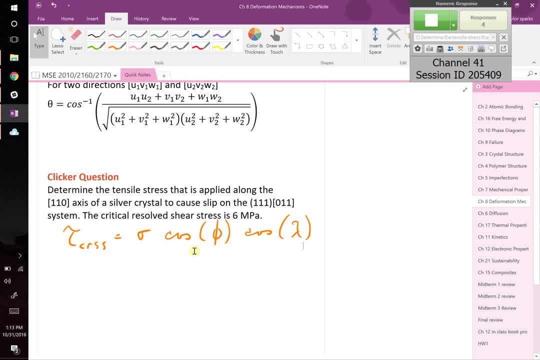 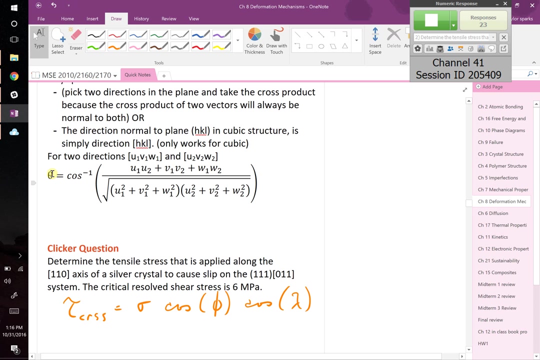 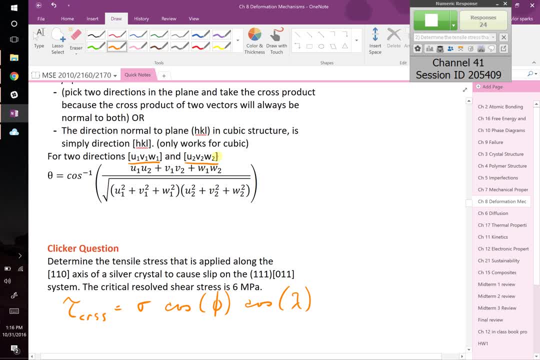 If you have vector one right here and vector two right here, theta is just the angle between any two generic vectors, right? So you plug in vector one and vector two. so, for example, this might be your loading direction And this one would then be maybe your normal to slip plane. 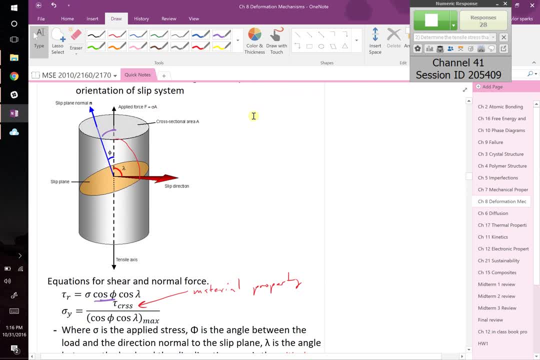 And if you do that, then you'll get one of the angles that you're looking for. You'll get the, then you get phi. You'll solve for phi, right? Then you do it again, but this time instead of slip plane. 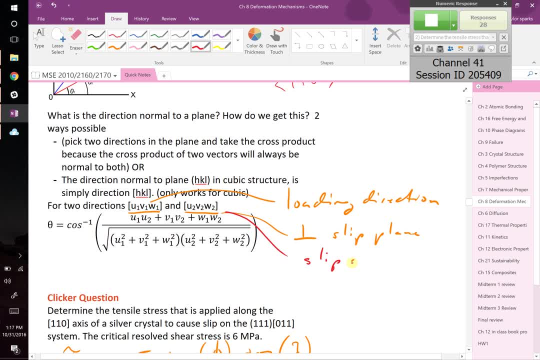 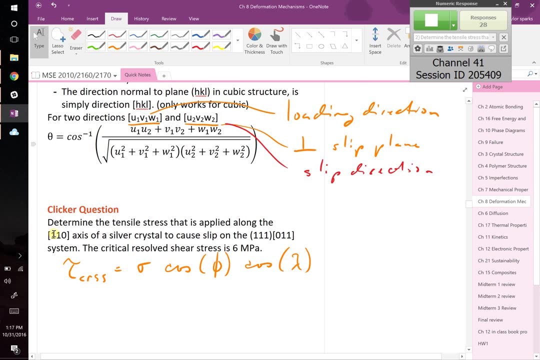 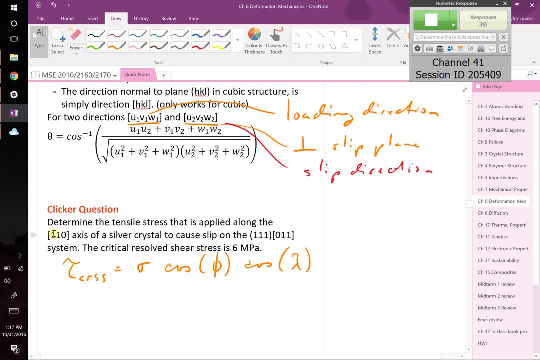 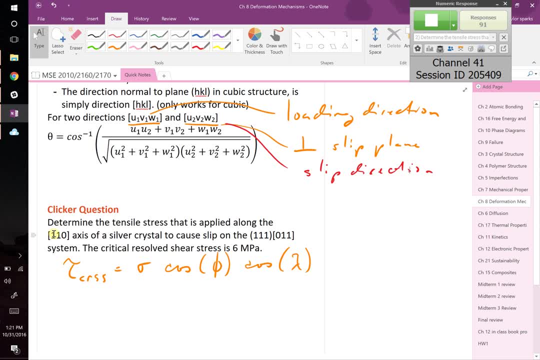 so we're going to give it a little more time on this. Your answers should be: ballpark 14-ish, Some right, So keep working. We won't stop just yet. Thank you, Thank you, Okay, can we wrap up? 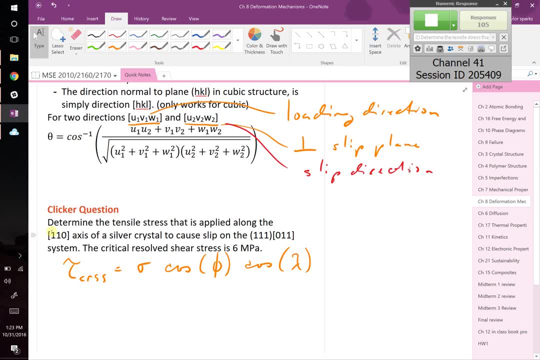 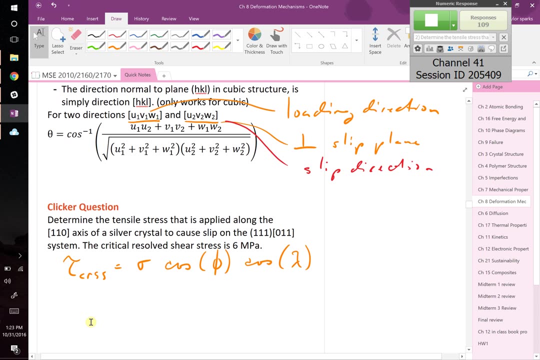 Let's do like one more minute. Get an answer in Phone- a friend, if you gotta At 24, we'll wrap up. Okay, we're going to wrap it up. Get your answers in, Okay. Okay, we're going to wrap it up. 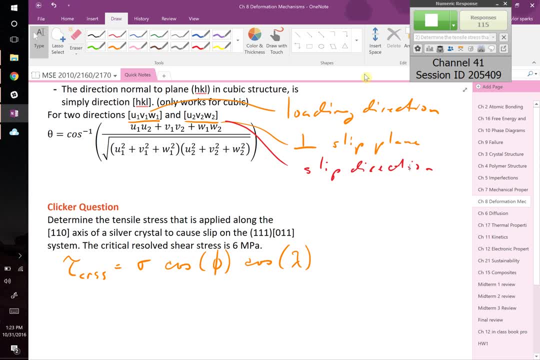 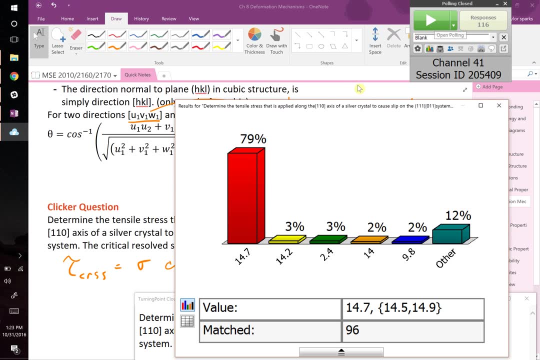 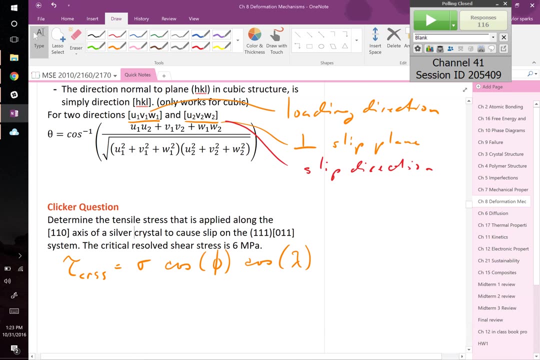 Get your answers in. Can we end? I'm going to end. Okay Answer's in. Okay, good, Most people got the correct answer, which is 14.7, right, So let's actually work through this together. So I told you. 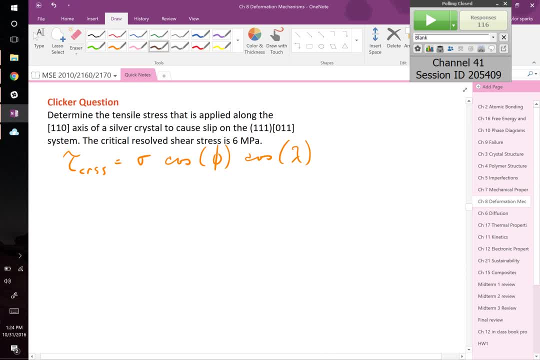 in the question that the resolved shear stress- which again that's a materials property, This thing, whenever the resolved shear stress hits six megapascals, this thing's going to start to slip. So the point at which it hits it, it's going to be the stress that we're 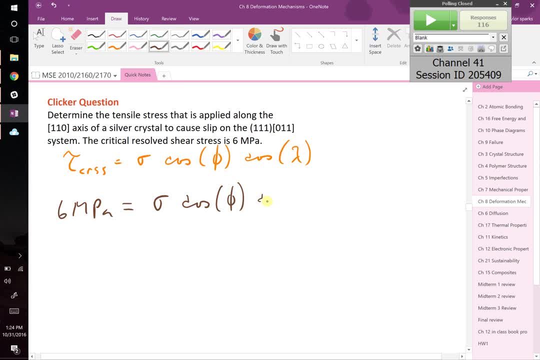 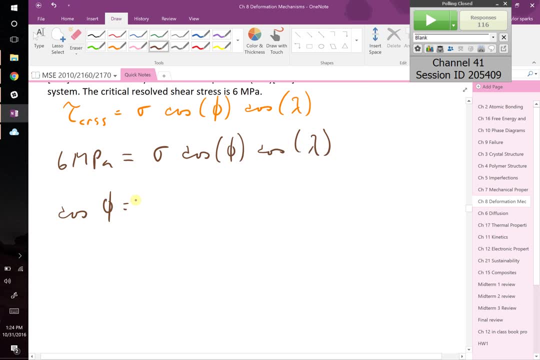 solving for times cosine of phi, times cosine of lambda, right. So let's do cosine of phi first. Cosine of phi is going to be equal to a dot b over the length of a over the length of b right. So again, the two angles here that we're talking about for phi, and it doesn't. 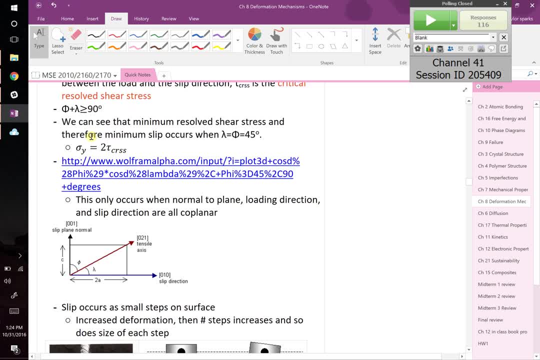 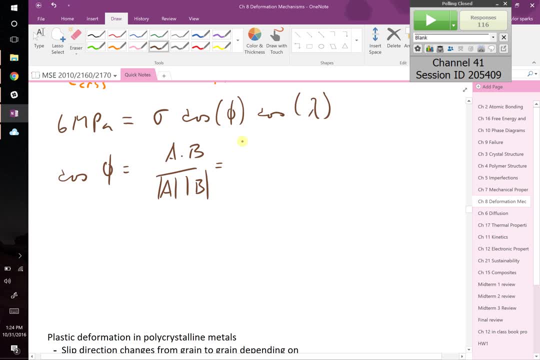 matter which one's which, but phi, technically is between the loading direction And the slip, normal. So that's between, that's the dot, between, excuse me, one one oh and one one one. And then here this is the length of the one one oh. 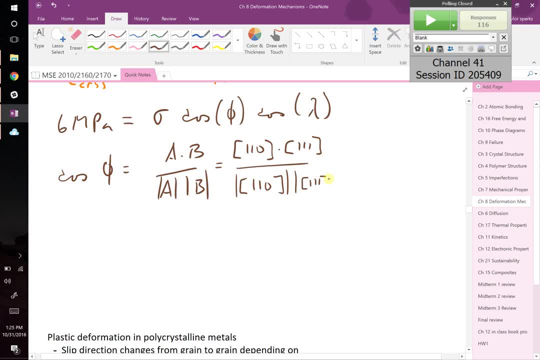 I guess we say the length of that and the one, one, one. When I do that, I find that that is equal to two over square root of six. Right Now, what's great is you don't actually have to solve for the angle itself is because 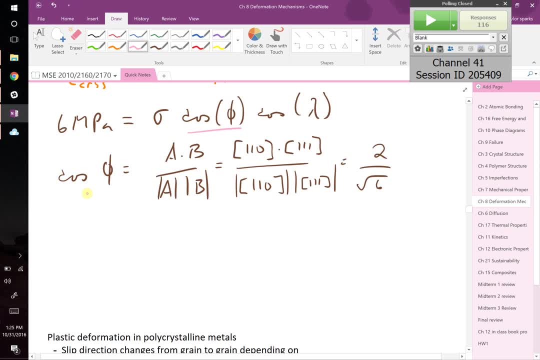 in this equation up here. all it wants is the cosine of that. we just solve for the cosine of that, So you don't actually have to plug in the angle if you don't want, save yourself the mathematical step there. So let's do the next one. So, cosine of lambda. 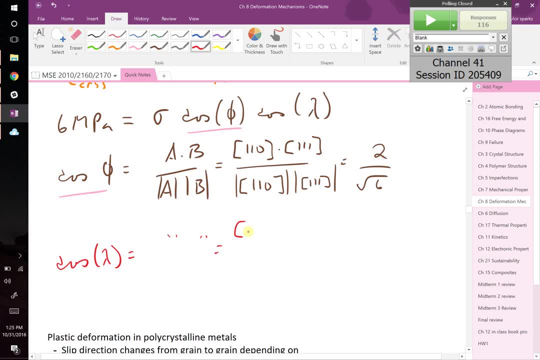 Again same equation, but this time it's going to be between one one oh and oh one one. So we're taking the length of the one vector and the length of the O and one vector. when I do that, I get one over. 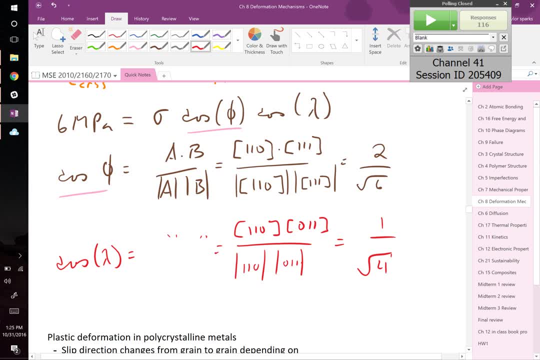 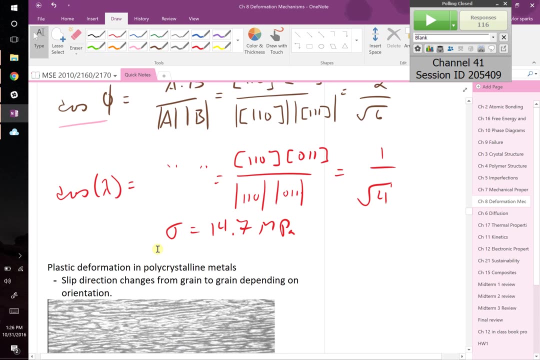 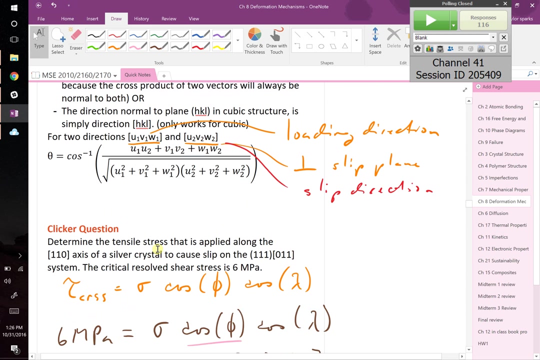 square root of four. right, so plugging in, I solve, for stress should be equal to fourteen point seven mega Pascals. okay, any questions on how we did this? any confusion at all there? yeah, so I gave it to you in this question. obviously, a question like this will be on the next midterm, for sure, I always use one. 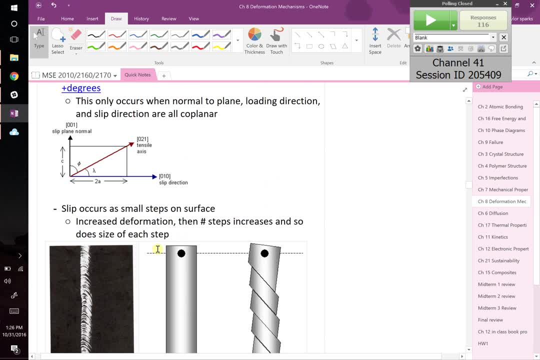 because there's lots of ways I can ask questions around it. right, I can say I would do this on a midterm because you wouldn't have time, but on a homework question I could say this: this resolves shear stress, and this loading stress caused slip to occur. what slip system might have been involved and you'd have? 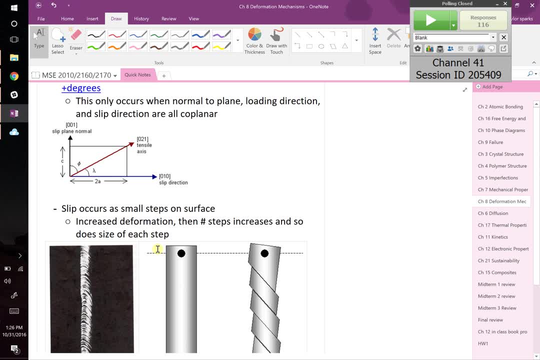 to guess at what the slip system might be, so I'm not gonna do that on a test. that would take too long. that's a reasonable thing on a homework though, because it'd be. if I said it's an SEC crystal, then you know that the slip system has to be the one-on-one. 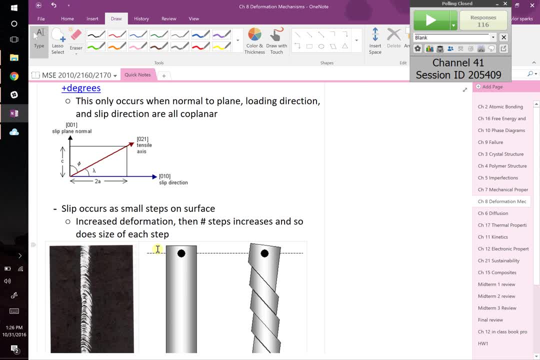 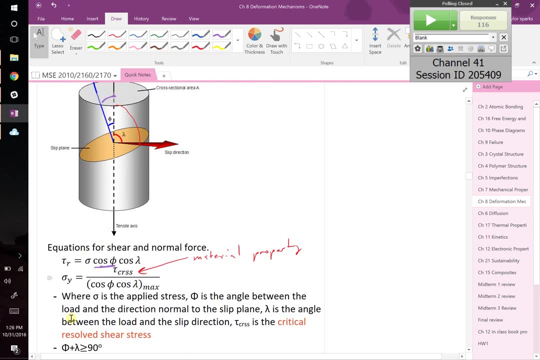 plane, so they don't have to do is figure out which direction it happened on. so you'd set up a little Excel spreadsheet. it wouldn't actually be too bad, right? so there's lots and lots of ways to ask these questions, because all it is is it's one formula, but it has to do with some vectors, right? so this tests whether 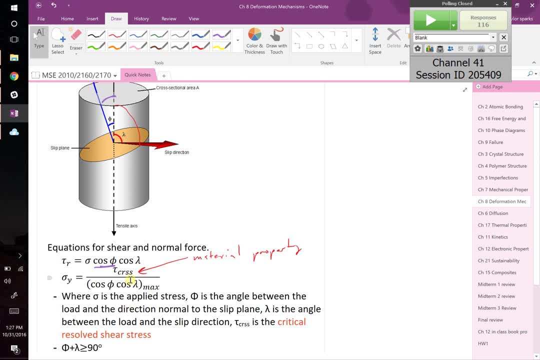 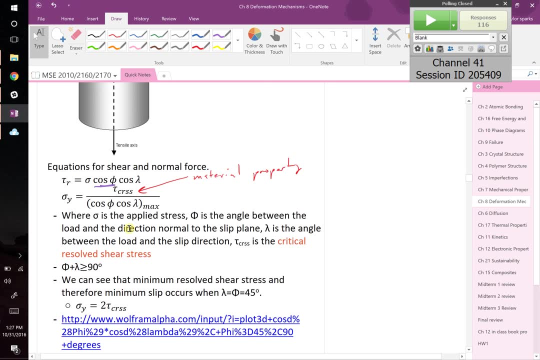 or not, you understand vectors, it understands. whether you understand, like plain Miller, indices and notation. you know the curly versus square, versus whatever brackets, right. so lots here to cover any other questions on it. that I that you was unclear about anything else. so again, the vector, the two vectors or the two angles we care about are always the loading. 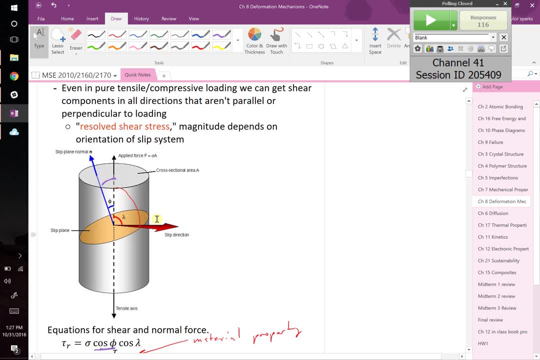 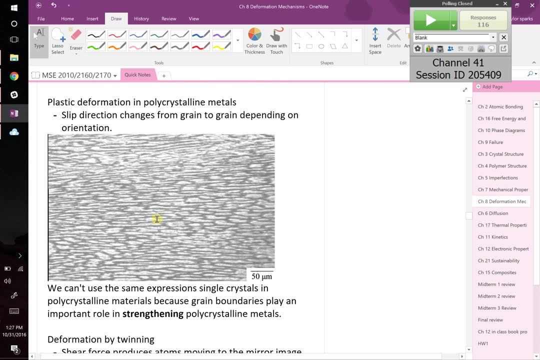 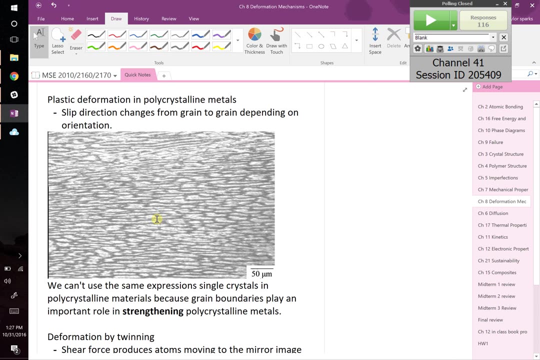 direction and the normal, the loading direction and the slip direction. right, those are the two angles we have to figure out, and they're actually not so bad to do. okay, so plastic deformation is different in polycrystalline materials. this equation is pretty handy, right, but it only works for single crystalline. 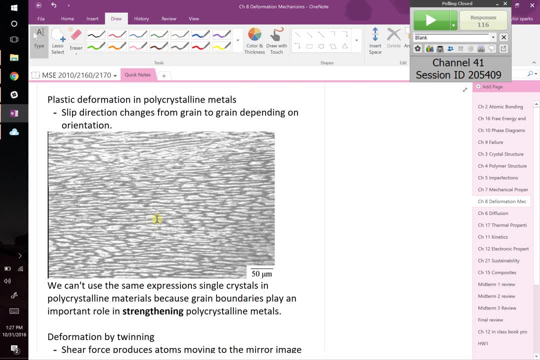 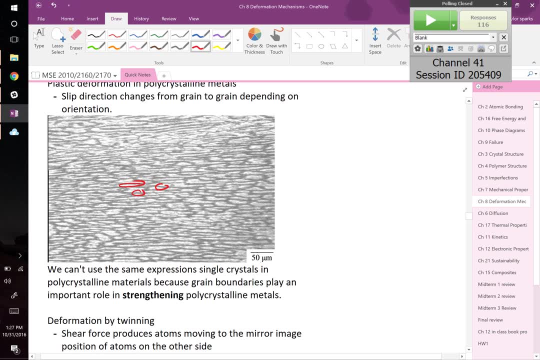 materials. right, because in polycrystalline materials we have the problem that every single one of these little domains here is a different grain boundary, it has a different orientation, and our equation depended on understanding the orientation of the crystal right. so, in fact, the strength of 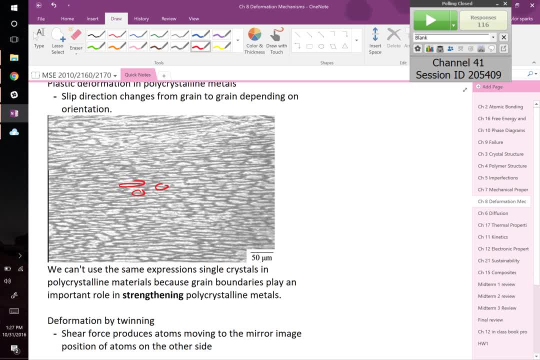 polycrystalline materials is going to be stronger than single crystalline materials because, let's say, you have a dislocation present right here and you know you're pulling on this thing in such a way that this thing wants to move that way. well, when it gets to a grain boundary, 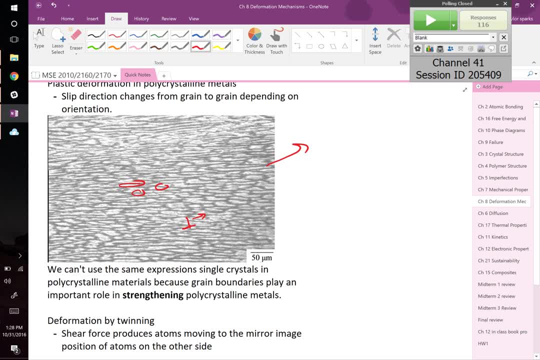 because the orientation of the adjacent grain is going to be different. it's going to have to redirect its direction a little bit. maybe it's going to have to move to, like that, to move through the next grade. so every one of these grain boundaries serves as a scattering site or a resistance of that dislocation to. 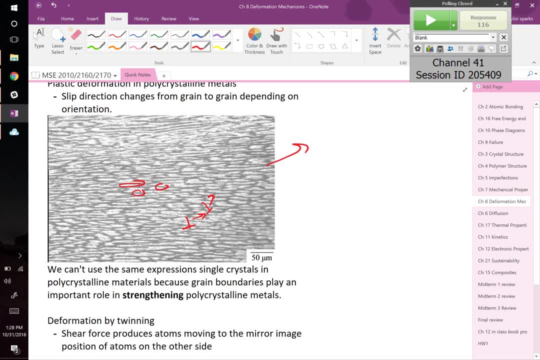 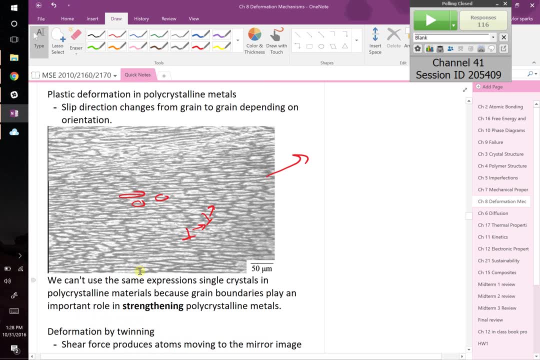 try and move through the material. therefore, the more grain boundaries you have, the stronger your material right, and this is actually a pretty common tool. this actually gets to help. etch in a minute that if you can just introduce more and more grain boundaries and use smaller, smaller grain materials, it'll get. 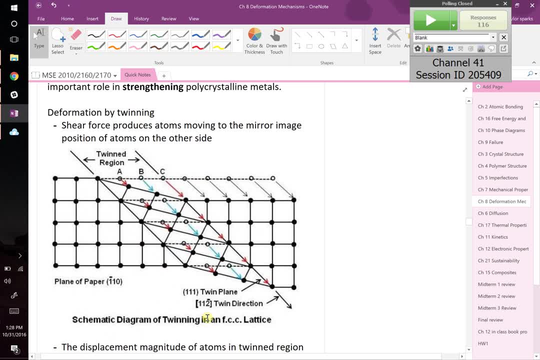 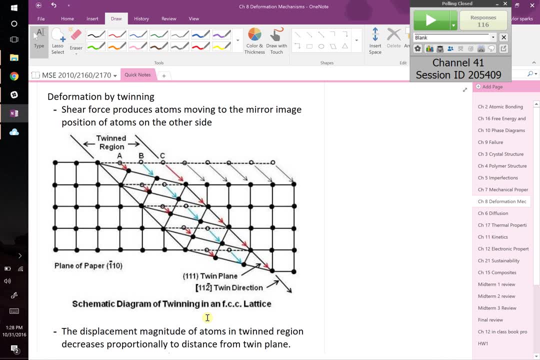 stronger and stronger, okay, okay, before we talk more about that with health pitch, let's talk about deformation by twinning. so if a dislocation can't move through a crystal, maybe because it doesn't have very many crystal slip systems right or because grain boundaries are causing problems, you can 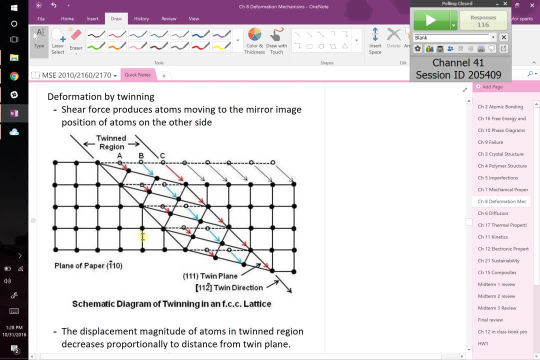 have twinning occur, right. so twinning- I think we mentioned this, that a shear force, right, so they're applying a force this way, in that way, so they're shearing it. it causes a collective motion of atoms right in the shear, or that, sorry, the twinned region or the shear region. okay, so that's what we call a shear force. 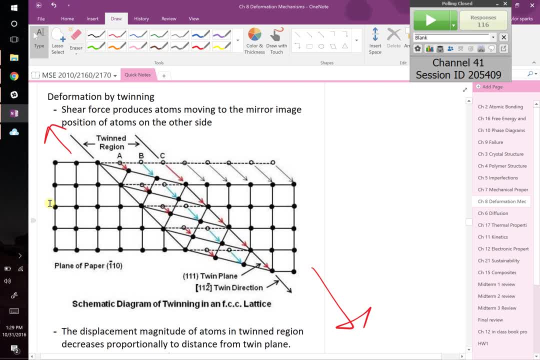 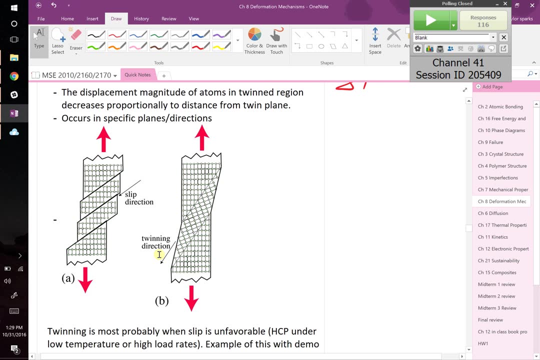 this picture is not strictly correct, because a twin should always have mirror images on both sides. and that's not quite mirror. it's off by a little bit, but it's pretty close, okay. so twinning can also occur. so both of these mechanisms can both produce deformation. right on the left we've got slipping occurring right and in here- remember, in the slip. 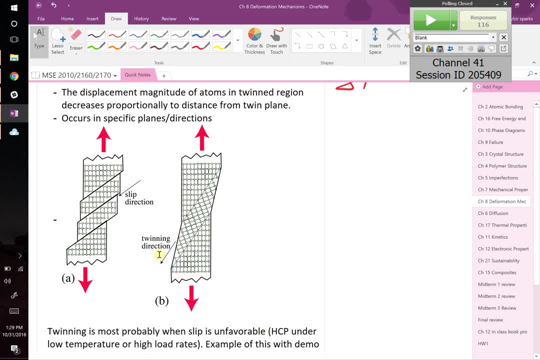 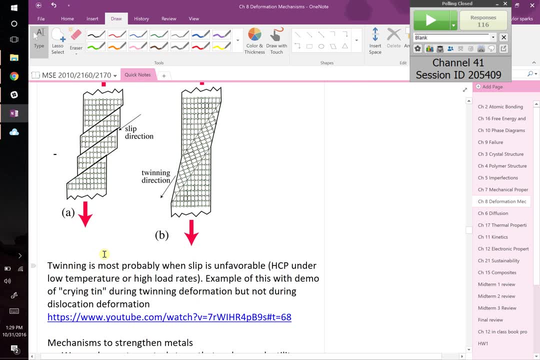 case the orientation is preserved throughout our single crystal. but in this case the orientation is not preserved. but we can achieve deformation by both roots right. so twinning will be more favorable or more probable if the slip system is unfavorable. so if you can't have slip, you'll 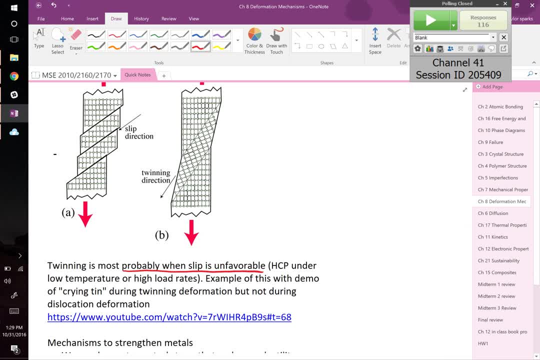 take twinning, and that's exactly what you see with the tin cry demo at the beginning of class. right in the first case, at room temperature, she took this piece of metal and as she bent it, you could hear it crackling. what do you think that crackling is? is it slip or is it twinning? 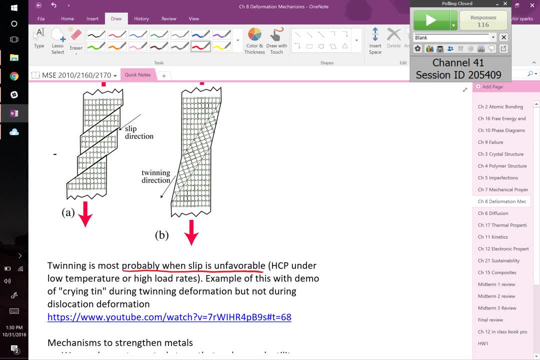 okay, what would make noise? what do you think should make noise slip? or twinning? so twinning is cooperative motion of many atoms. that's a sound wave. right, when a bunch of atoms shift, that creates a sound wave. it's a pressure wave that would then go through the material. so twinning. 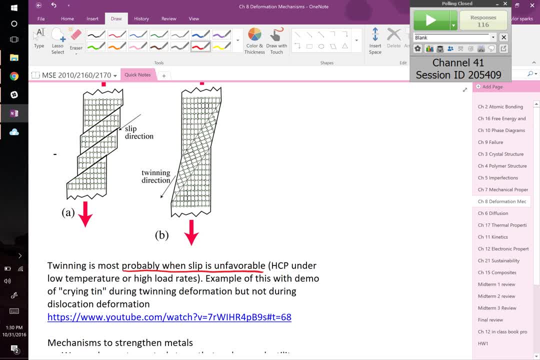 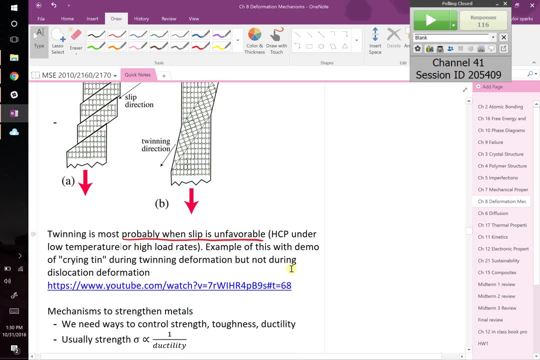 creates, uh, that crying, that crinkling noise. that's literally the, the shift of atoms slip doesn't have that because it doesn't have as many atoms all shifting at once, right, yeah, so crying occurs during the twinning deformation, exactly right, like at winter warm. you can see this, uh, because the energy of theрp temperature. 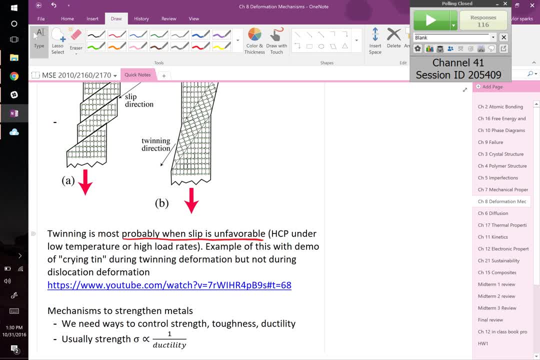 is long, it heats it up and it places where the energy is. but then, when we heat it up and we give it some thermal energy, all of a sudden, the more favorable mechanism is slip, and so it's able to deform, be a slip, and you don't get that, that crying motion of the collective motion of atoms. 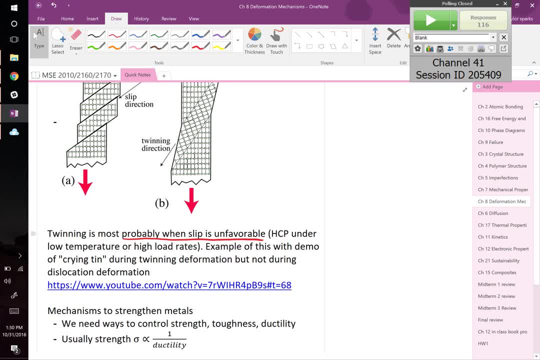 okay, any questions on that? yeah, so it seems like, um, when it was eating up after, after it was bent, it seemed like it still retained, like most of the strength, but when it's slipping it seem like great segue into the next section. So hold that thought. We're coming to that. What as you deform? 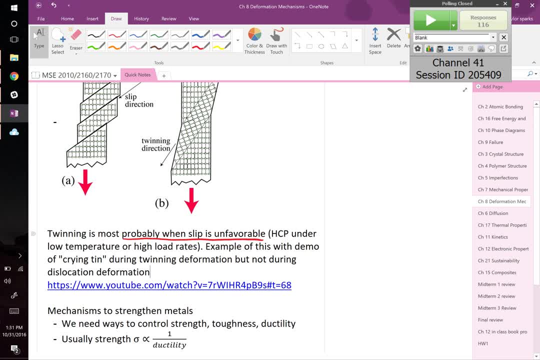 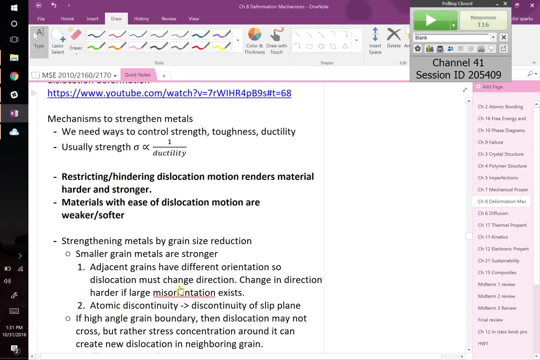 these things. what does it do to the strength is really the heart of the question there, So let's come back to that in just one second, Okay? So first off, when we talk about all these mechanisms of deforming or strengthening of metals, there's always a trade-off. You can never have it both. 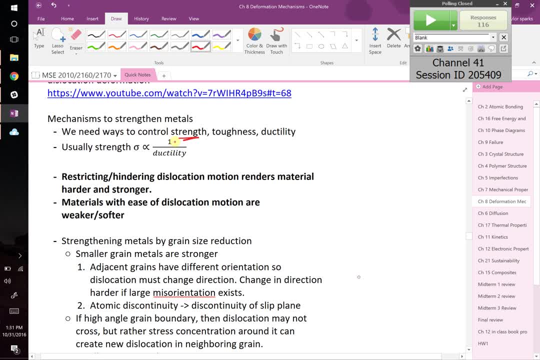 ways. If you want to increase your strength, then you lose toughness and you lose ductility, right? So this is like your general trade-off: Increasing strength comes at the expense of ductility. If you want more ductility, you have to lose some strength, right? And the reason why that happens? 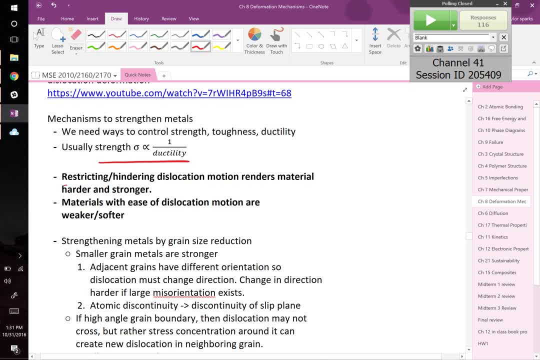 is because- this next point here- that anytime you restrict or hinder dislocation motion, you render the material harder and stronger. If you make dislocation motion easier, you make it weaker and softer. So the blacksmith takes his piece of metal and he puts it in the forge and 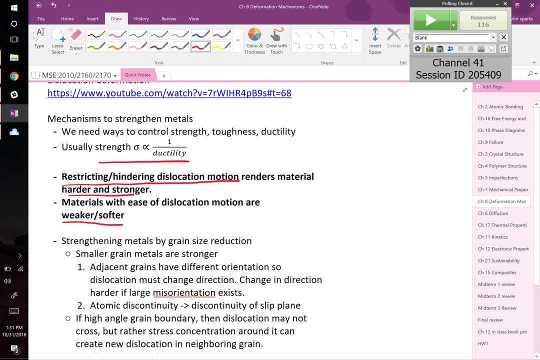 gets it glowing hot And now all of a sudden it's easy to deform. The reason it's easy to deform is because you gave it a ton of thermal energy, So these slips can move past each other a little bit here. So you can see that it's easy to deform. So you can see that it's easy to deform. So you can. 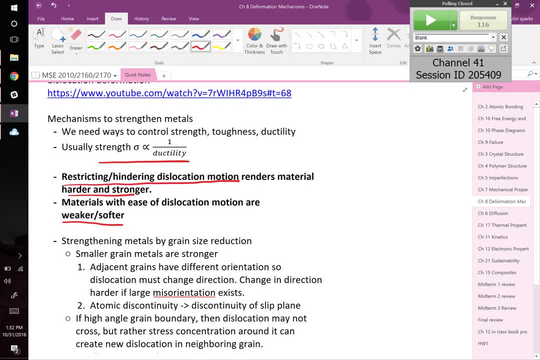 see that it's easier, right When it cools down, it gets harder and stronger, because those dislocations can't move past each other- one another. So this is a really important take-home message for material scientists, mechanical engineers alike: If you do anything to make it, 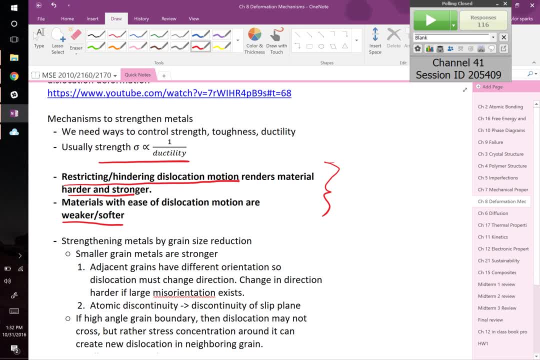 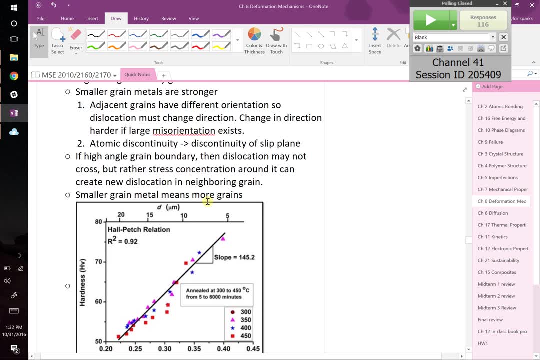 harder for them to move. you made a harder, stronger material, but you've sacrificed ductility, right? So we mentioned that reducing grain size will strengthen a material, And it does that exactly because grain boundaries serve as scattering sites for dislocations. So you can. 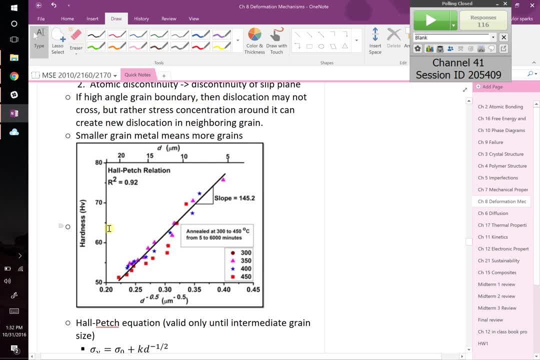 see that there's sort of a linear relationship. If you were to place a piece of metal on a piece of metal, you're going to have to plot the hardness or strength. hardness against the inverse square root of grain size, right? So here's the actual expression: Your yield strength. 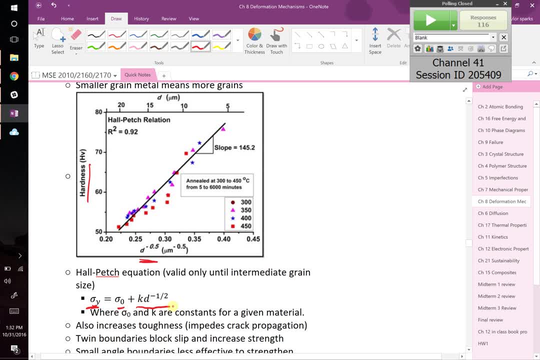 is going to be equal to some minimum yield strength plus KD to the negative one-half. where D to the negative one-half, that's your grain size to the negative one-half. So plotting here: that's what they're plotting here, right, They've got D to the negative one-half. 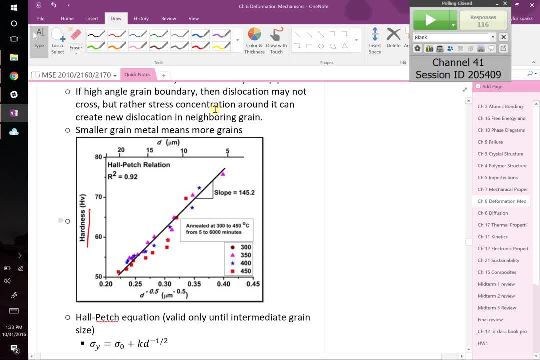 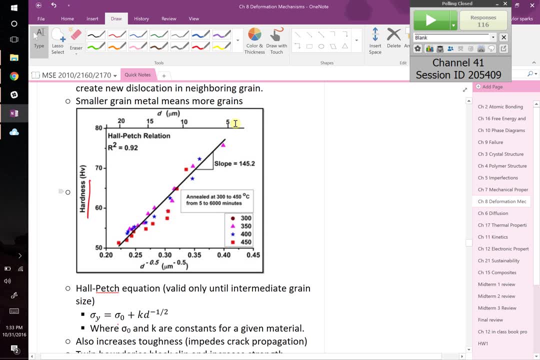 here. So basically, small grains- yeah, small grains- and hardness, Large grains. You see, your small grain material is much harder, like a factor of 50% or 75% higher hardness. okay, And this is simply because dislocations can't move. So because this is nice, 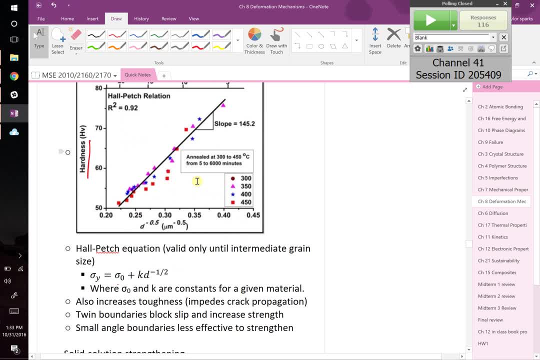 and linear over a nice range, we can actually fit it. And that slope will give us K, which is going to be well, K and your sigma naught, those are your Hall-Petch constants, right, Which is great, because if you have 316 steel and they say how strong it is, well, it really depends on how big. 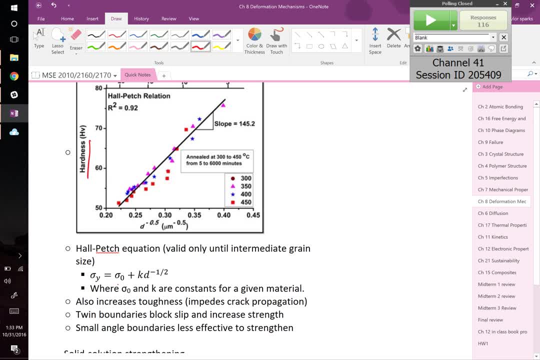 it is right. So it's not useful for them to say like, hey, this 316 steel is such and such a strength. They should really say what the average grain size is right, Because then you're going to know why it has the strength it has, And it's going to be due to this Hall-Petch equation. 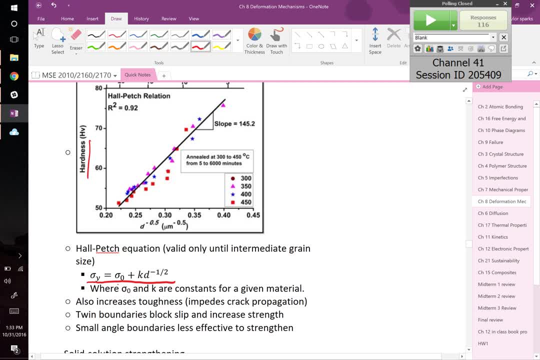 It also means that if you do something to your material that has small grains to cause them to grow, which we'll get to in a moment- you're going to weaken your material, right? So if you're planning on using something at high temperatures or some temperature where you're going to see, 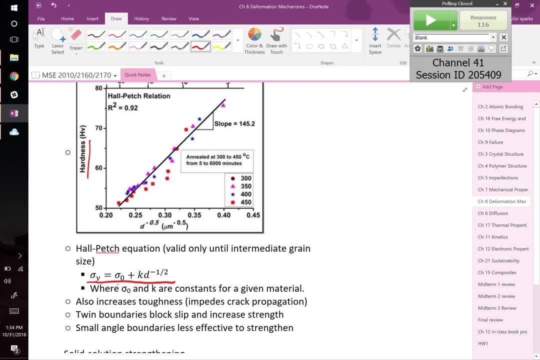 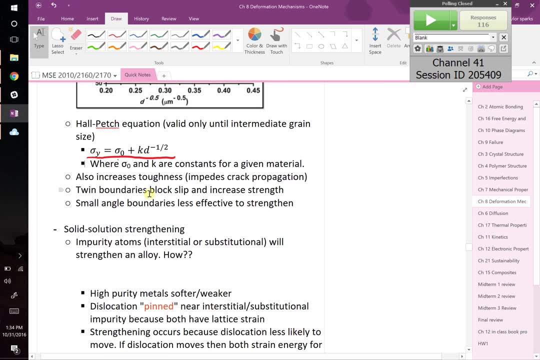 grain growth. don't be surprised if your strength goes down from what the spec sheet says, basically right. Also, as you go to smaller and smaller grains, therefore more and more grain boundaries, you increase toughness because you impede crack motion as well. It's not just dislocations that. 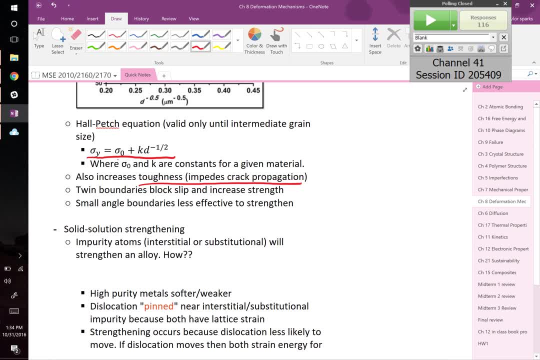 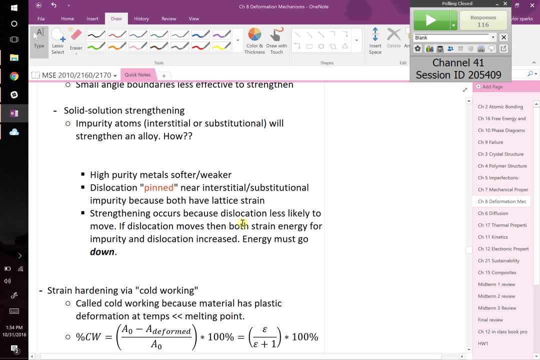 can't move, but whole cracks get blocked by grains, right, So you increase the fracture toughness. Okay, Solid solution strength, And we've said this a couple of times in class now- but like, sterling silver is the great example of this, Start with pure silver. 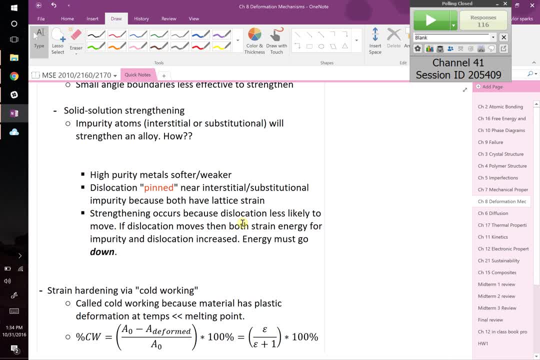 add a little bit of copper, Since copper is not the right size. it has a strain field around it. Therefore, dislocation is going to want to hang out with that copper atom and it's not going to want to move. If you made a dislocation harder to move, you strengthened your material right. 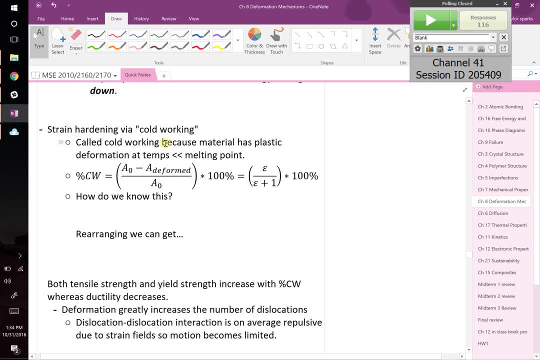 Okay, Strain hardening or cold working. They call it cold working because as you plastically deform something, it's typically lower than its melting point that you're doing this, And if you do it much below its melting point then you're not constantly fixing all the damage. 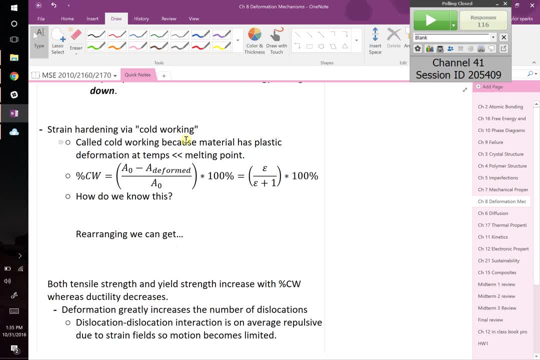 you put into it. So if I take, this is my piece of metal, Every time I pound on it I introduce dislocations into it. If this is at a low temperature, those dislocations can't reverse and heal themselves and annihilate. therefore they're. 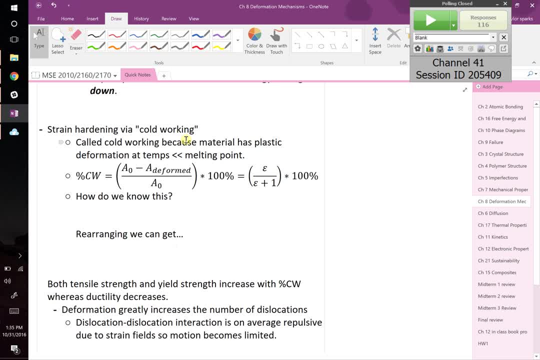 still there. Therefore, every time I hit this with a hammer after I've there's, I'm just adding more and more dislocations and they start to resist one another right. So if you don't ever fix that, it's just going to get harder and harder and more and more likely to 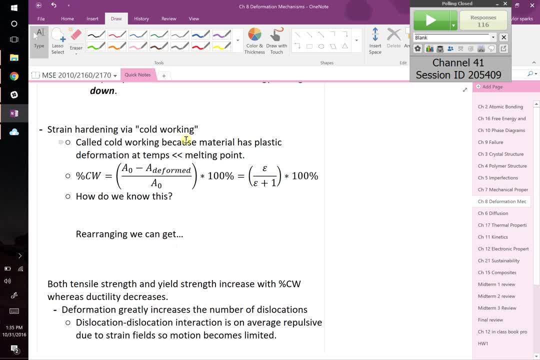 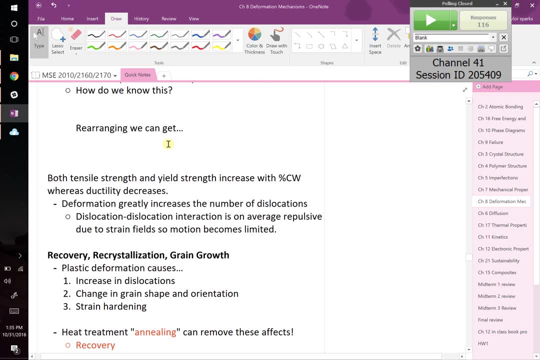 fracture, which is why a blacksmith can't just keep on hitting his piece when it's out of the oven, because eventually it's just going to fracture. Okay, We'll skip What is cold working. Why use it? Great question. Okay, So now we have two ideas. One is to avoid using a blacksmith because it's multiple pieces. 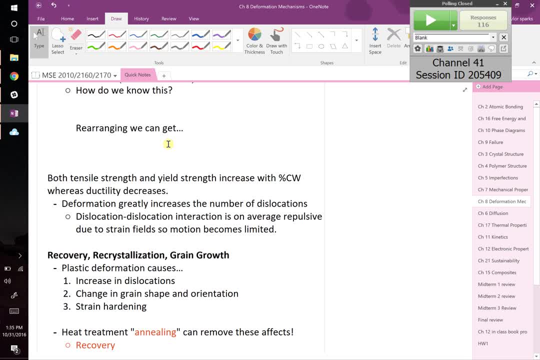 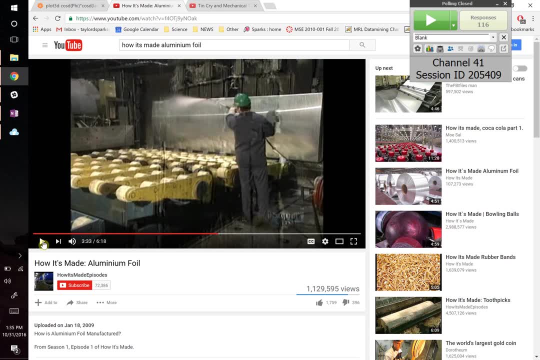 great question. why would you want to use cold working versus hot working? by the way, hot working- did they actually use it? they absolutely do. here's a. there's a picture of how it's made. my kid loves these, so take a look at this. this is how. 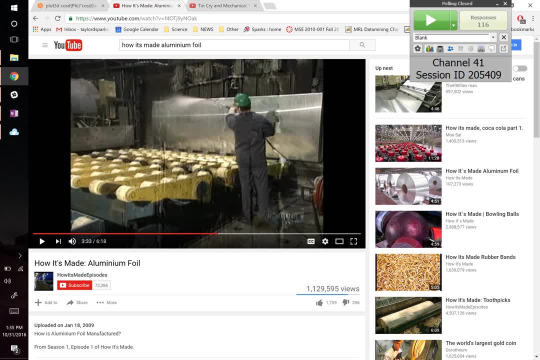 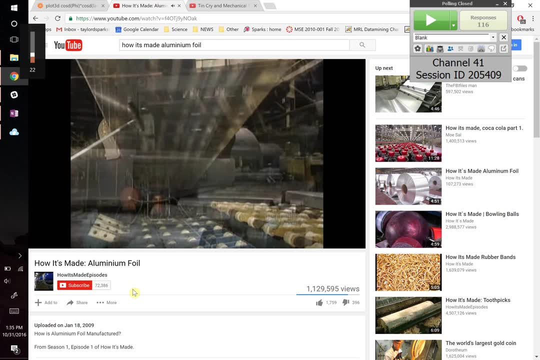 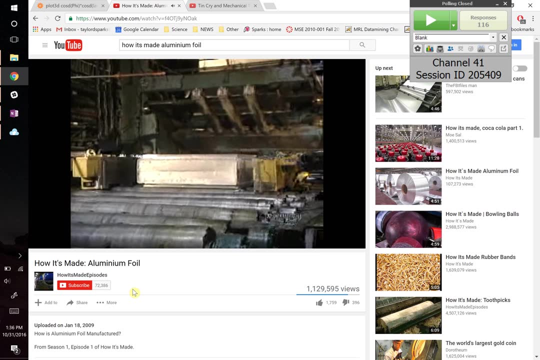 they make. aluminum foil, believe it or not, starts out with thousands of pound giant ingots of all traces of the liquid used to cool the decrusting knives have to be eliminated, so they cast the ingot first. then what do they do? the many steps in the thinning of the ingot begins. 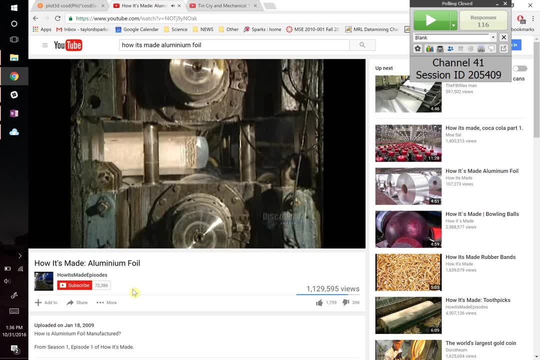 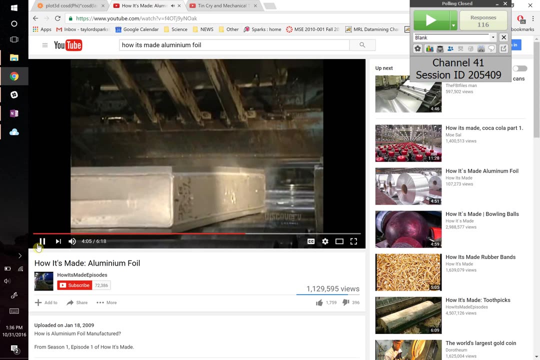 the aluminum block is crushed by the hot mill rollers. temperatures in the rollers are between 455 and 540 degrees. centigrade pressure on the ingot is continually verified by a technician. if too great, it's lowered and the technician then adjusts the pressure. the heat is 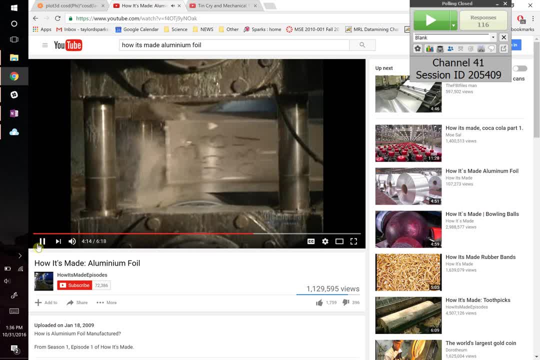 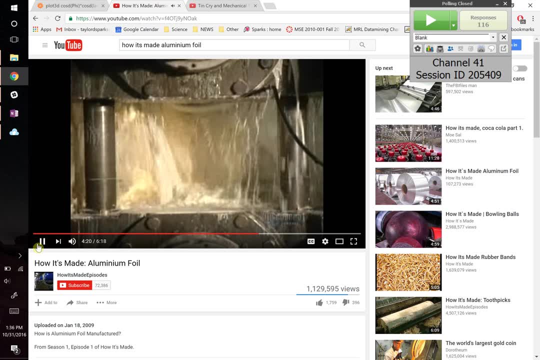 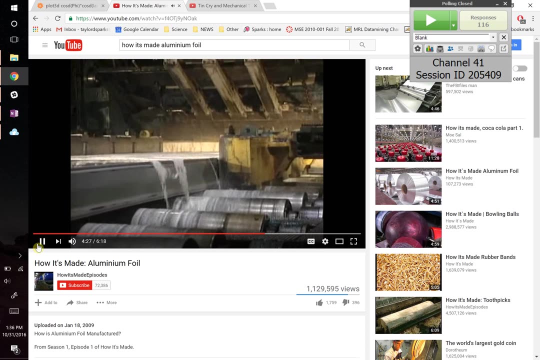 so high that the ingot risks sticking to the mills roller. to prevent this, everything is cooled with a liquid that's 95% water and 5% oil. they have to have that oil so it doesn't stick to the rollers itself. the ingot. they do this over and over, starting from a thickness of 45 centimeters. the ingot. 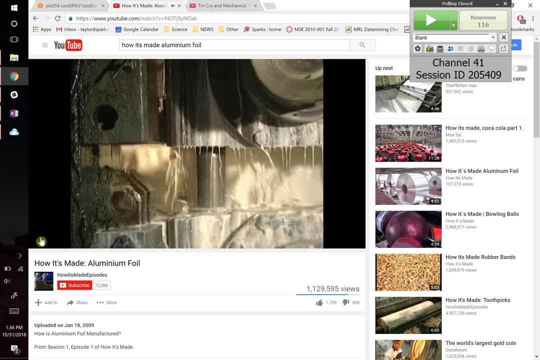 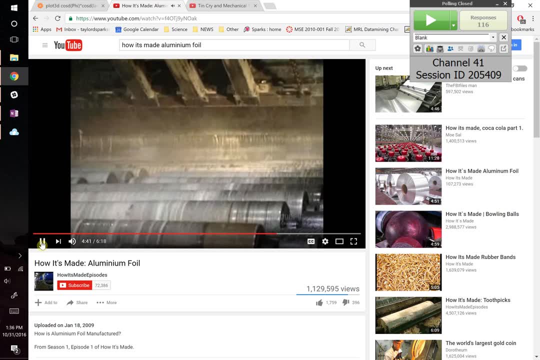 becomes increasingly thinner with each pass through. depending on requirements, the ingot will go through the machine between 12 and 16 times. the ingot will be casted on the machine between 12 and 16 times. the ingot will be casted on the machine between 12 and 16 times. 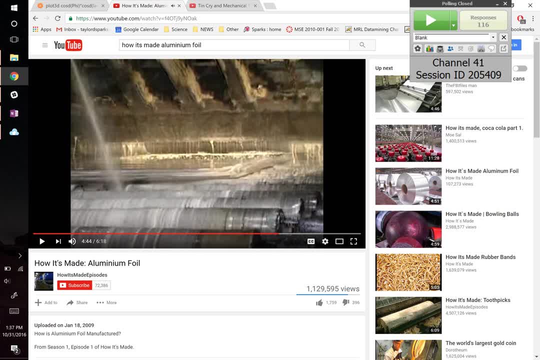 the ingot will be casted on the machine between 12 and 16 times. so it's clear why they do it at high temperatures. right, it's just easier and it's constantly healing out the deformation so it's less likely to fracture. so why would you ever do cold working, meaning you're deforming it at? 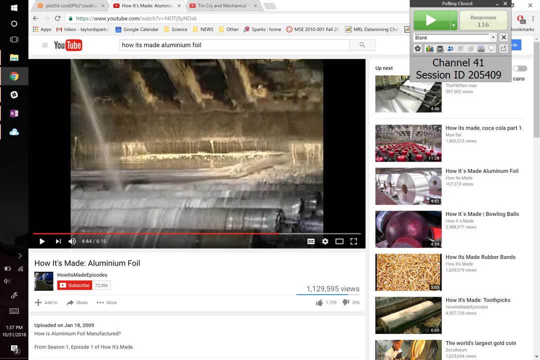 low temperatures. any ideas? yeah, Eric, yeah, you can say the same thing, Steve. yeah, if you want your final foil to be more stiff, mean it's more likely to break, but a higher strength, especially in the in the rolling direction. yeah, you could just do a cold working right. so for a lot of applications they do do that and it produces. 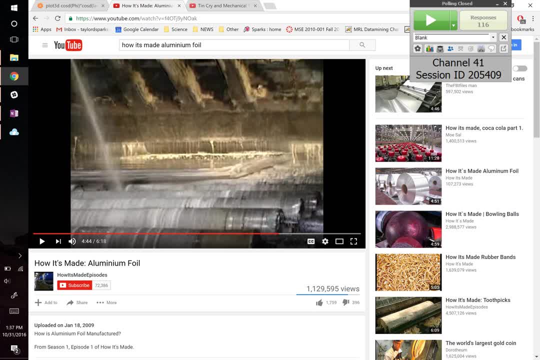 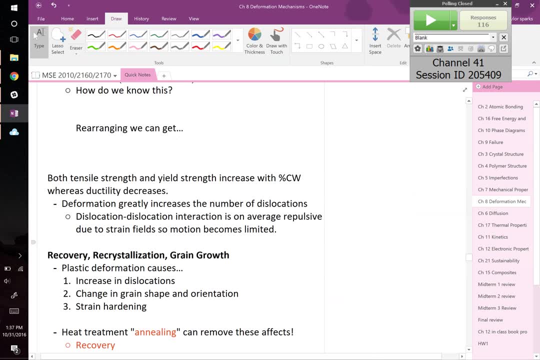 a stronger. so maybe, like for your final pass, it's too weak because you've been doing it hot, but your final pass you might do that one cold to give it some higher strength. okay, matt, you also have a lot. sure, anywhere where you do cold working you're going to make a more brittle area and if you 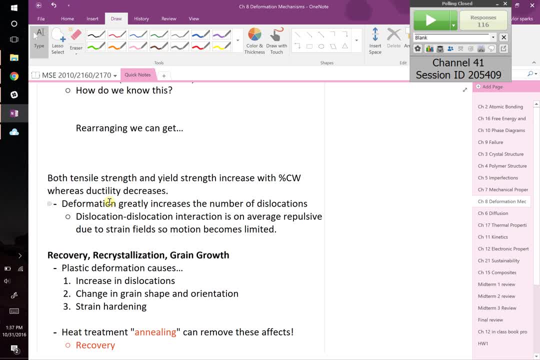 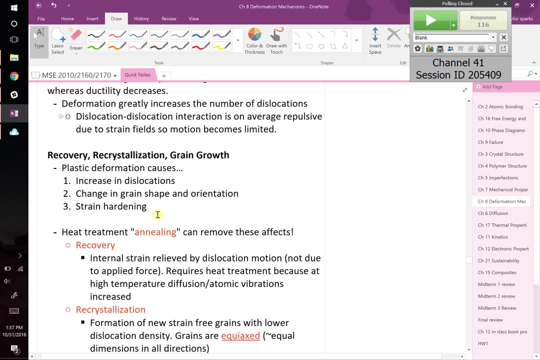 wanted to then use it as like a design feature where now it's going to break specifically along wherever you did the cold working. yeah, absolutely okay, okay. so all this talking about introducing dislocations, getting rid of them, having it become harder, having it go back to more ductile can be. 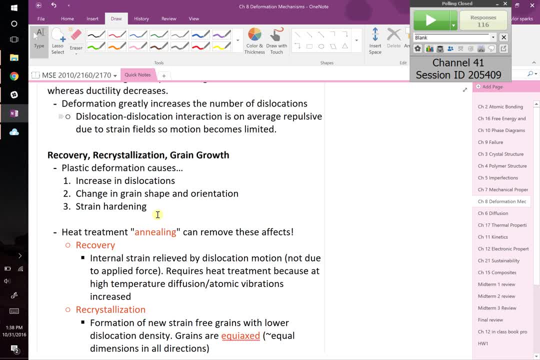 described in terms of words, of using material science, called recovery, recrystallization and grain growth. right? so we already said that plastic deformation causes more dislocations. it changes the grain shape and the orientation, right? so this is here. right, if you start out with like normal. 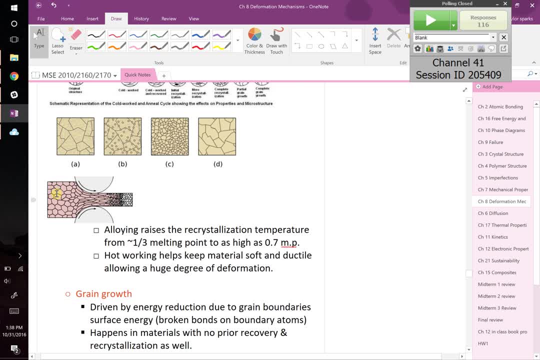 equiaxed grains. equiaxed means you're going to have more dislocations and you're going to have more creeps and you're going to have more 옆учey affect the structure. this is kind of thick balancing. you're going to have more corrective. 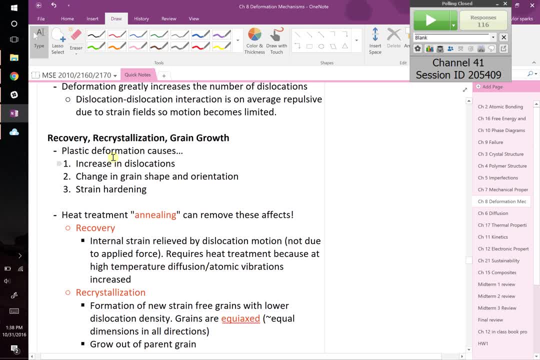 digitization break down everything and we don't avoid this. we want to start off with some change in the shape of the grain. it's adapted. the way we anticipate it may be different. you have particles adjoining them when there's no adjoining principle, so you're sometimes seen 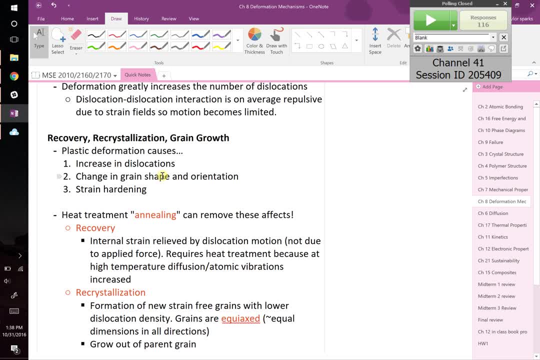 on thezedog and you're in the same situation where you get therooms and the headstreet and this is where we place too much into the point that we want to haveологy to introduce a more working it more and more likely to break and your final product: you don't want it to break, so they have. 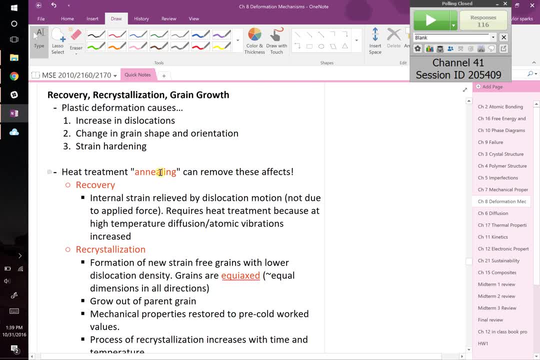 to recover those things right. so they anneal it, which is just a heat treating step meant to remove the effects caused by plastic deformation. they call it recovery as the first step because internal strain starts to be relieved, but relieved by dislocation motion, meaning let's say you had an 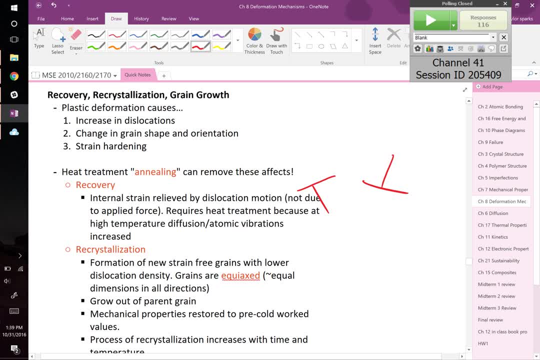 initial dislocation like that, another one like this: you add a little bit of thermal energy. this thing can line up with that one. they feel an attractive force, they combine and they annihilate. right, so it got better. right there was recovery. so that's the first thing that occurs when you 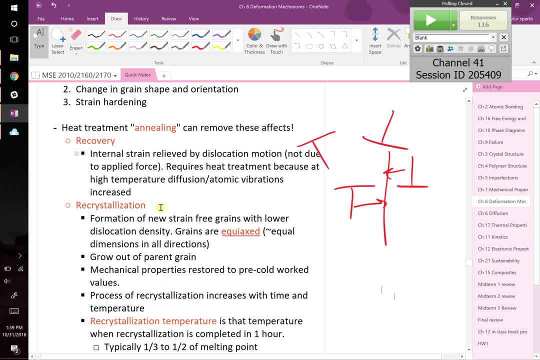 give it a little bit of heat during the annealing right. if your system is so messed up and it has so many dislocations and you provide enough thermal energy, your crystal might just say: you know what it's easier to start from scratch, like when i go in a room sometime and somebody's had. 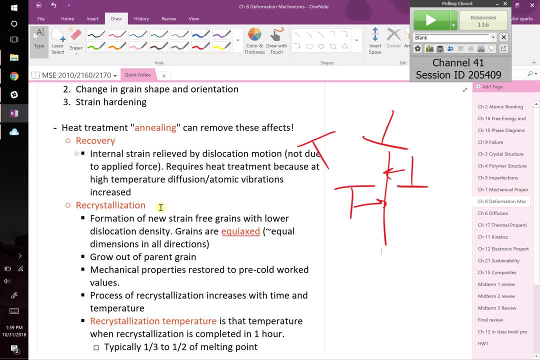 like the chairs like all over the place. sometimes, rather than trying to take the existing chairs which are all over the place and try and make a nice grid, it's easier just to push all the chairs to one side and start lining them up again in some sort of way. 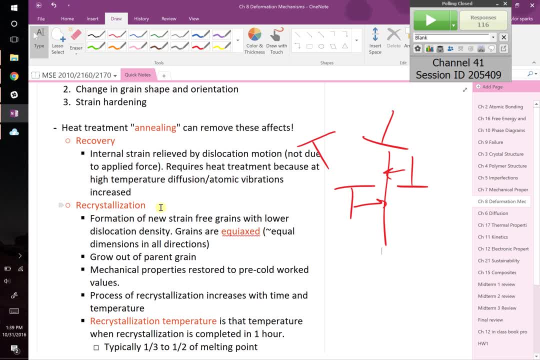 nice arrangement. that's the difference between recovery and recrystallization. recovery says: try and move the individual chairs to make it work within the existing lattice. recrystallization says: it's too broken, let's just crystallize new bomb or new grains. entirely right, so you form. 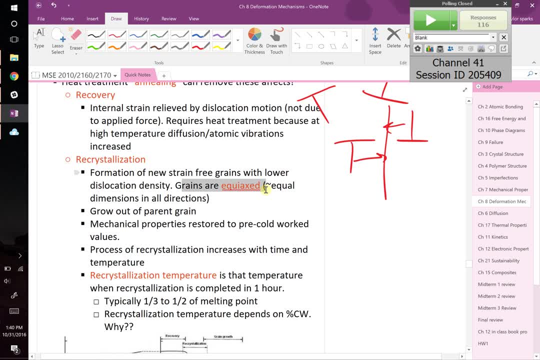 entirely new strain-free grains. these will be equiaxed, meaning that they don't have a preferred orientation. they're going to be random and sort of spherical shaped as opposed to long, and drawn out. maybe these grow out of the parent grain and then by doing so you get mechanical properties. 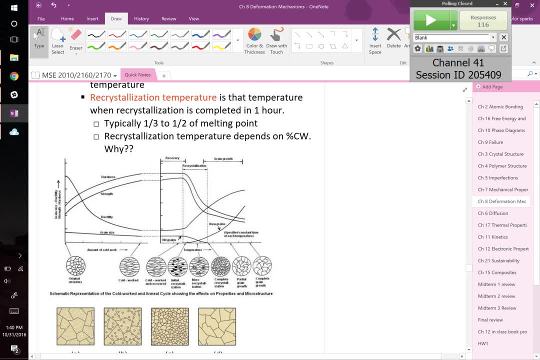 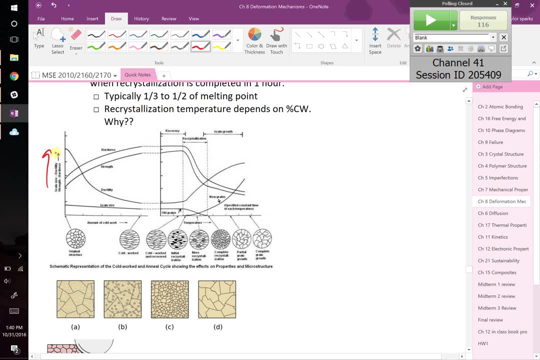 material. right so this is increasing ductility and increasing strength on different axes, right so that's either more ductility or strength. so, hardness as you cold work it, hardness goes up, but ductility goes down. right as you're cold working it, you put it in the oven and you start. 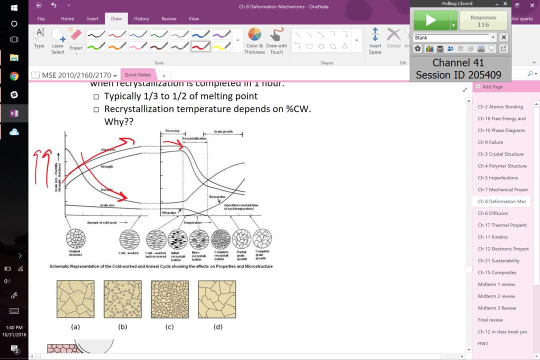 to get recovery and you're going to see moderate, very small changes to hardness and very small changes to ductility. a little bit, though by the time you get into recrystallization your hardness is going to plummet right and your ductility is going to really take off to kind of 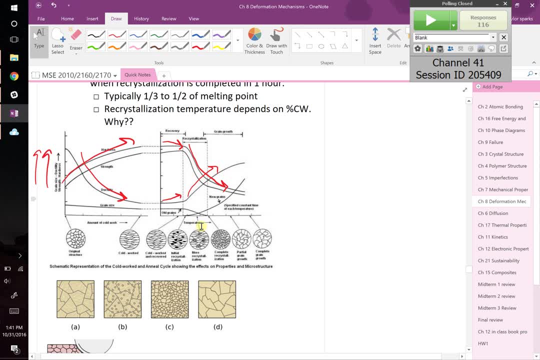 where they were when you started, right. then the last step is grain growth. right, so you started out growing these tiny new little strain free grains, right? so here's our, our new grains, starting to crystallize, right, recrystallization, right. so those are new strain free grains. they're not stretched. 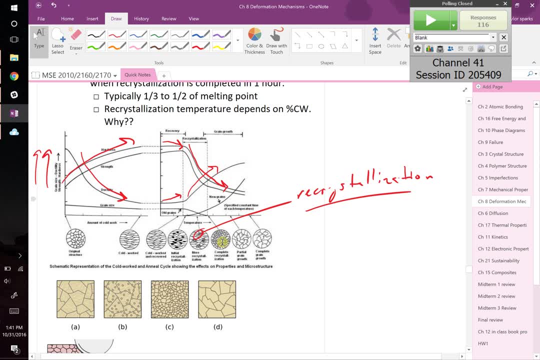 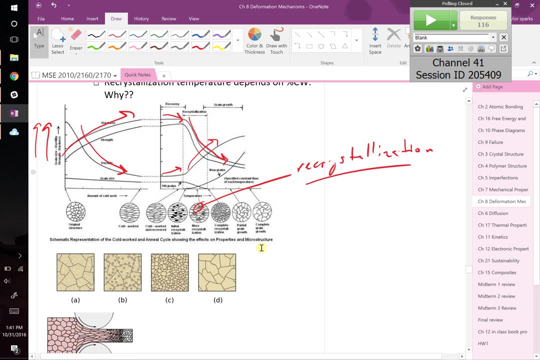 out. they're nice and equiaxed, they grow, and then you've got a whole bunch of them. once you've gotten rid of all the old grains, what you're going to do is you're going to take a little bit of the broth out into form. we call it this: two wheat, gift or water will sort of come together in natural. 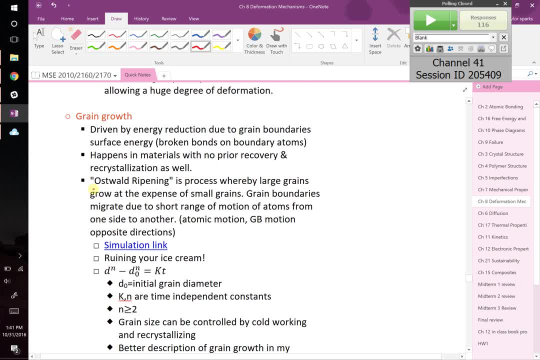 reflection of the new grains that you're growing, right. so if you leave this at high temperatures for a while, these small grains will grow into large grains, and the reason that happens is due to something called oswald ripening. the book calls it awesome ripening. all that means is 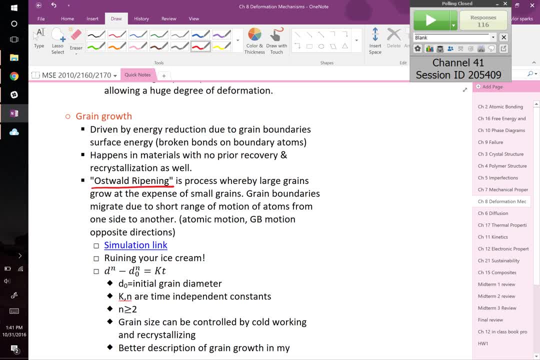 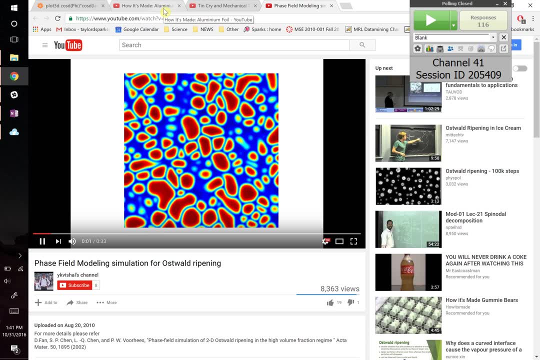 if you have small grains, those ones get swallowed up and big grains swallowed, or the ones that swallow them. so small grains disappear, big ones get bigger. so if this happens and you let it go, computer simulation of a bunch of small grains and if they leave it at a high temperature, right? 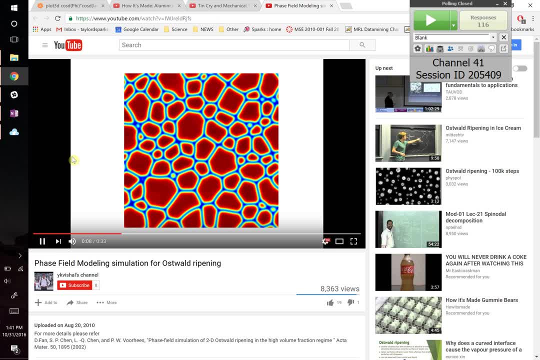 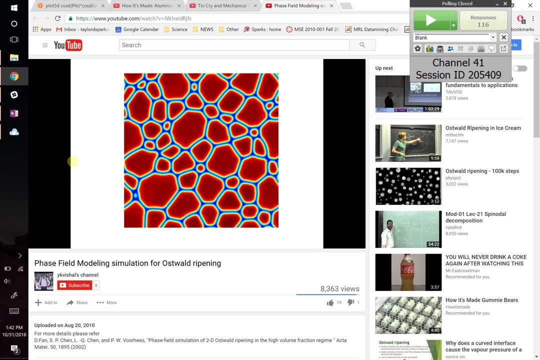 in the. in the model you can see that these small grains are getting eaten up by the big ones, so over time they're getting swallowed up. now, what's the driving force for this surface? energy. right, every surface has an energy. we don't like it, so we'd like to get rid of them. so it happens now. 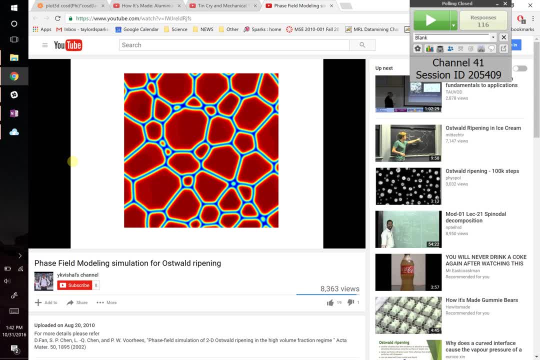 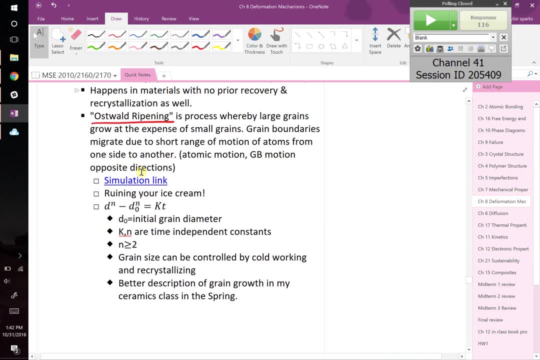 the mechanism we won't get into in this class. you'll probably learn in other ones. my ceramics, we talk about it, but basically big ones get bigger, small ones get smaller. it's a sad commentary on living life, right? and this is also what ruins your ice cream, right? actually, when you get, when 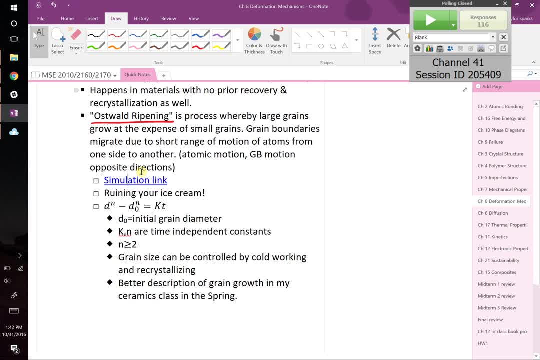 you buy ice cream from the manufacturer. it's quite small grain, which is delicious, right. but when you let this thing, uh, you take it out of the out of the fridge for a minute and you serve it up and then you put it back in. you expose it to a higher temperature, so you gave. 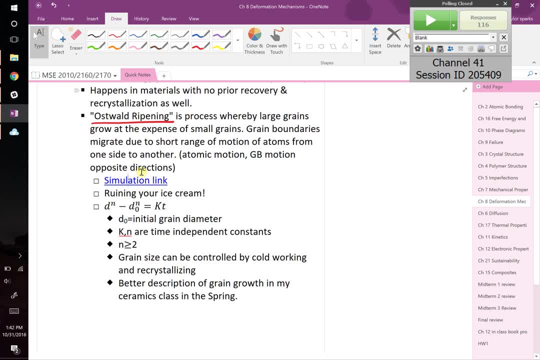 it thermal energy for those grains to grow and you also gave it energy for the cream and the water to separate. so when the cream and the water separates, now your ice crystal is there and it's not tiny and it's going to grow. and every time you do this, that ice crystal is going to get.